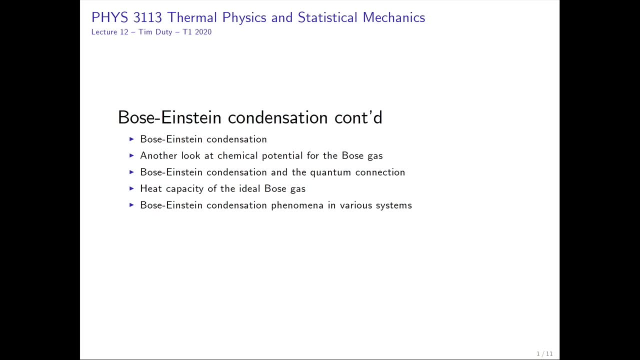 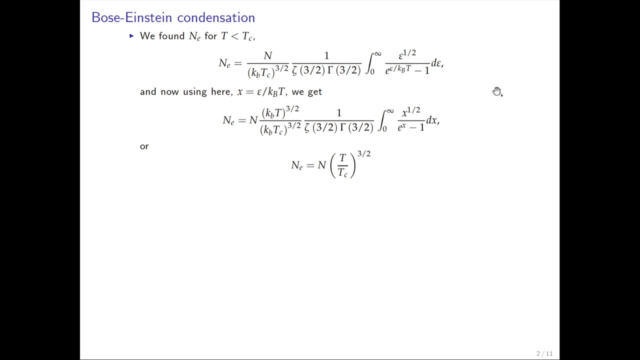 gas, and we'll discuss that. And finally, I'll talk about Bose-Einstein condensation phenomena in various systems. Okay, so let's get started. So last time we looked at the number of fermions- sorry, number of bosons in, not in, the ground- 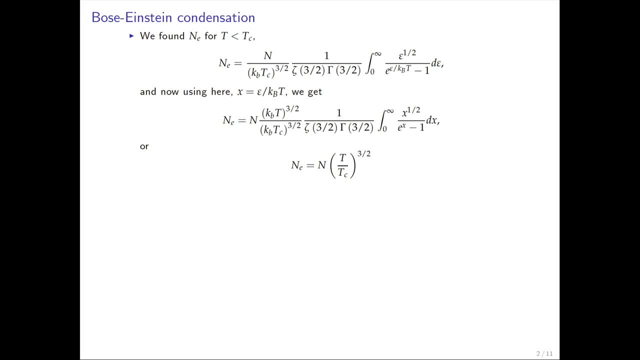 state, so the number in the excited states below this critical temperature that we derived before. And remember we got the critical temperature by imagining that we didn't have to worry about the ground state and we would try to maintain the total number of particles. 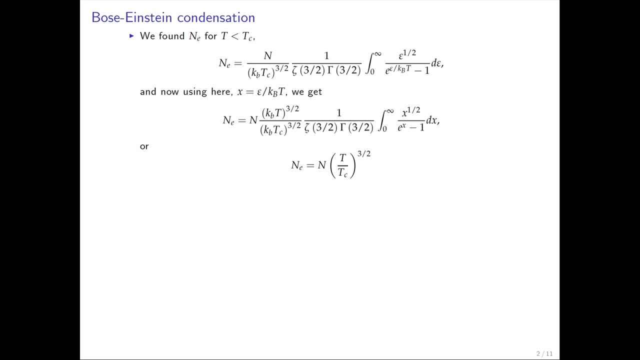 by adjusting chemical potential, and we found that that was not possible. So we looked at the temperature below the critical temperature, and so then we went back and we separated out the system into ground state and excited states And we realized: well, let's just. 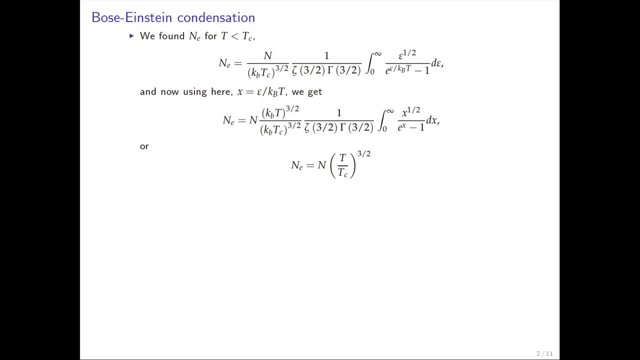 calculate, below Tc, what the number in the excited state would be, which will be less, of course, than the total number. And we do that just, of course, by this integral over the density of states. And we also remarked that, since we had already found the critical, 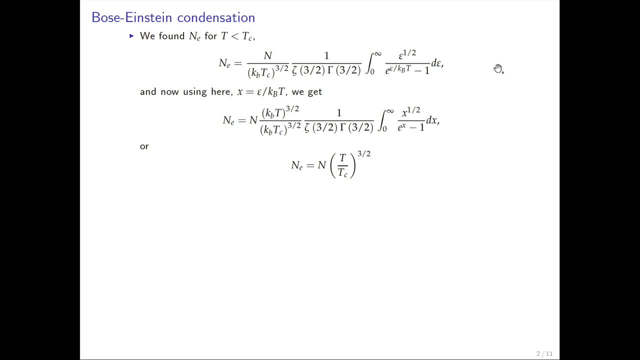 temperature. we could write the density of states in a more convenient form that involved the critical temperature, like we've done in the past when we studied fermions, and that gives the constant out front here, which is the zeta function and the gamma function. 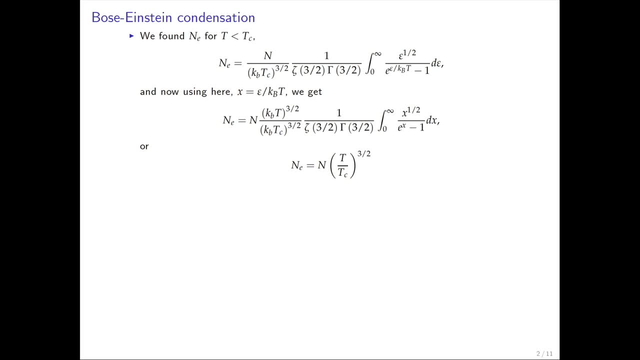 They're just numbers and we discussed what those numbers were in the last lecture, And so now we're going to look at this again: below Tc, some arbitrary temperature, T below Tc- and to find a number in the excited state. of course, this integral leaves out the ground. 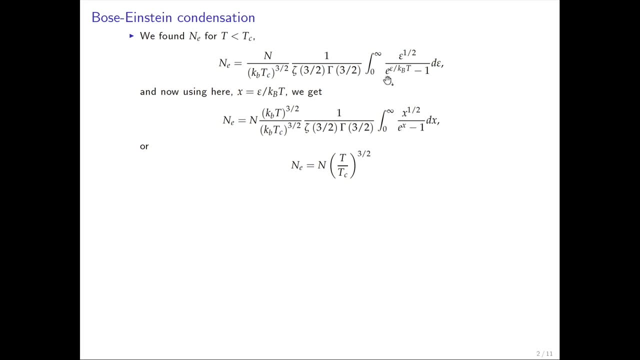 state at energy, epsilon equals zero, but we can find the number in the excited state this way and it will be less than of course, this factor will end up to be less than one, right? So? and when we do that? so we just look at this integral and this integral it's helpful. 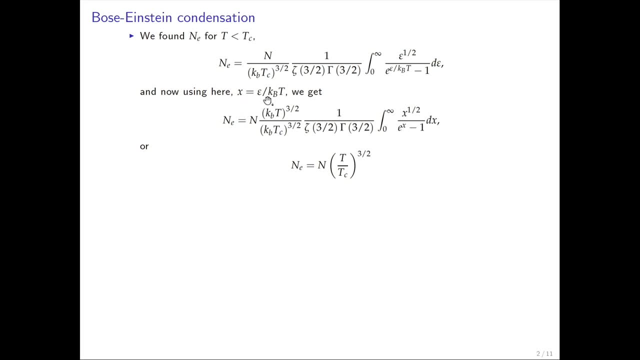 to change variables again to this dimensionless x, which is epsilon over kbt, and we did that sort of last time. we did all this last time, by the way, if you want, I want to review that again and we can complete this integral and, of course, this factor turns. 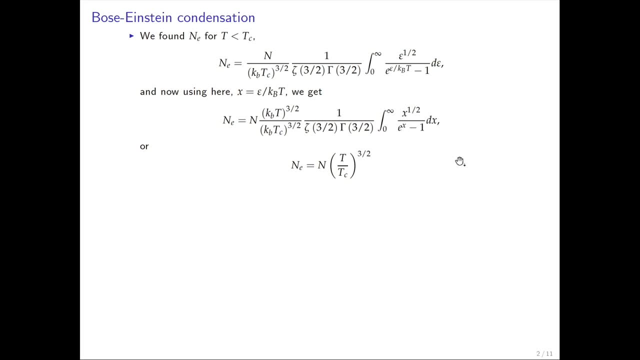 out to cancel out these factors, because we already did that before with finding the critical temperature and in the end we find that the number of particles in the excited state is n and, as we said, it must be some factor that's less than one and, of course, when T, 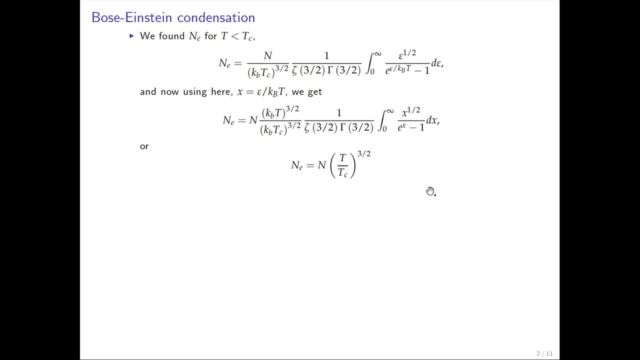 is less than Tc. this is factor less than one, and so to the three halves power, it will be less than one, And this tells us that there's. So, if we look at the fraction, which is the number of particles in the excited state divided, 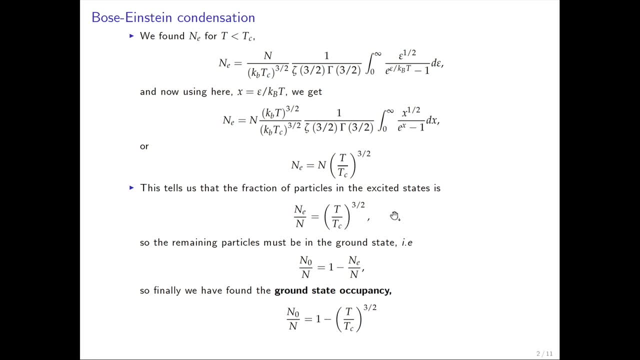 by the total number, it's basically T over Tc to the three half power, and so, of course, the remaining particles must be the fraction in the ground state, and that gives us then this equation for the ground state occupancy, or the fraction number of particles in the 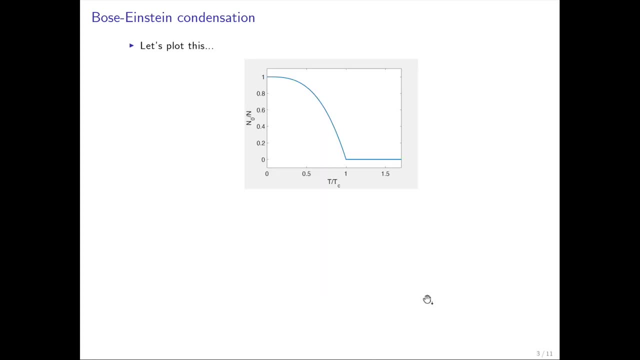 ground state that has this dependence, and we plotted that and it looked like this. it rises quickly from the critical temperature, It goes to one okay, And for T greater than the critical temperature, well, the number of particles in the ground. 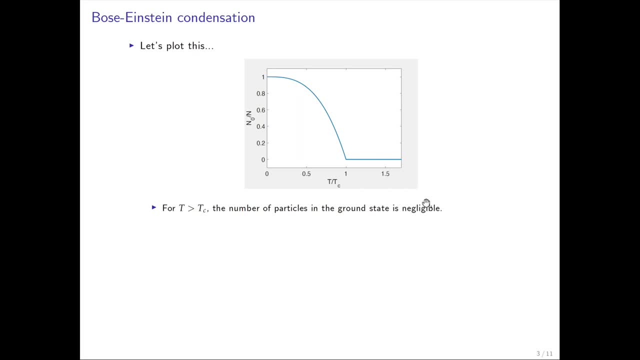 state is negligible and we don't have to worry so much. we can just use that integral to calculate that. But below this critical temperature, of course, as shown in this plot, the number in the ground state increases rapidly and this is a phenomenon of Bose-Einstein condensation and the way 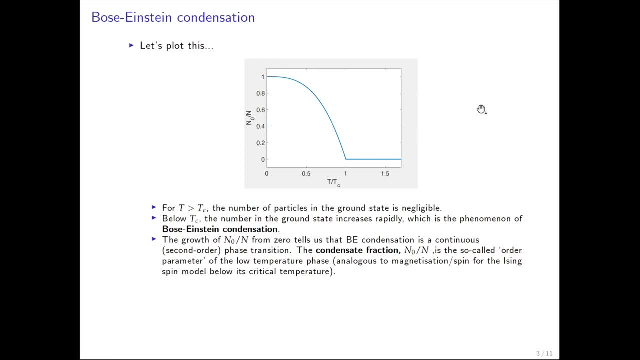 this grows. It indicates that it's a continuous second-order phase transition and this condensate fraction, as we call it, fraction in the ground state, is a kind of order parameter in this low-temperature phase. If you want to think of an analogy, you think about the magnetization per spin for something. 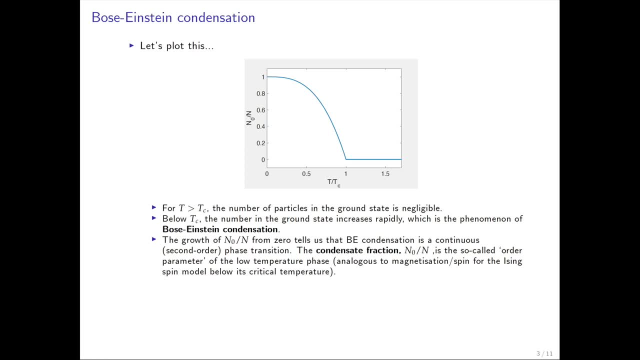 like the Ising model or some other spin model that grows below its critical temperature. that's the order parameter for the kind of spin model And this condensate fraction. Okay, It's a kind of order parameter of the low-temperature phase for this Bose-Einstein condensation. 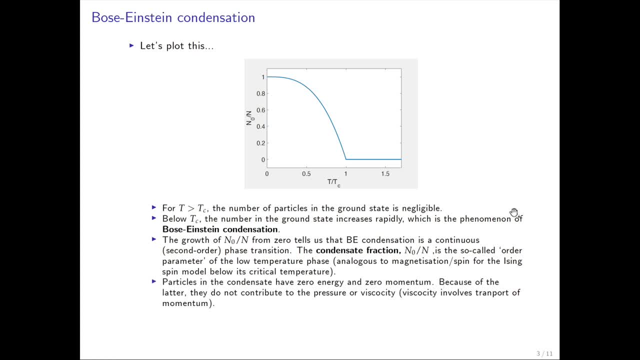 And we also mentioned that particles in the condensate have zero energy and zero momentum and because of this they don't contribute to pressure or viscosity, and we'll discuss this a little bit at the end of this lecture. when we talk about superfluid helium-4, which 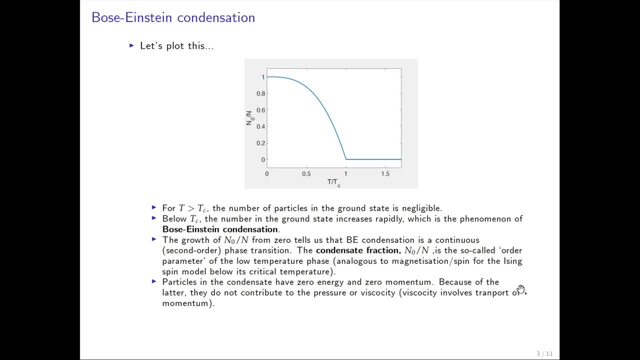 has zero viscosity, because it's a type, It's a kind of Bose-Einstein condensation, at least in my opinion. Okay, It's a kind of Bose-Einstein condensation, at least approximately. And yeah, and also I mentioned last time that Bose-Einstein condensate it's not really. 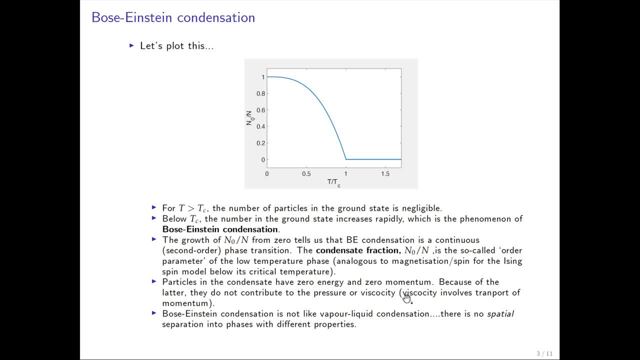 like a liquid, so much It's a very special kind of condensate and there's no spatial separation in the phases with different properties. So it's not like in a liquid gas that if you have a container and you have this condensation. 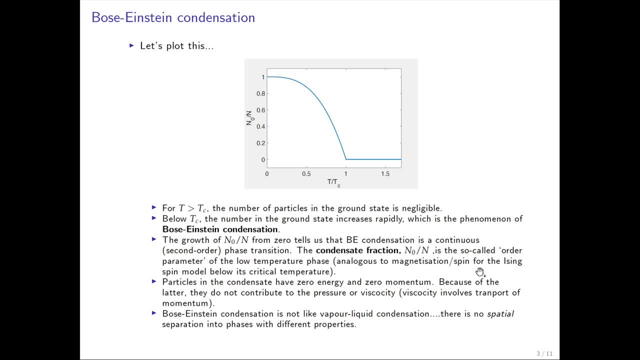 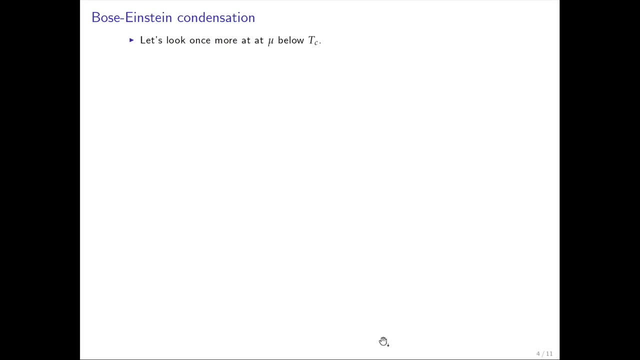 you have the liquid sitting somewhere At the bottom of this vessel and the gas around it. it's not like it's all intermixed, of course. Okay, So let's. So. that was all from the last lecture and I just wanted to review it. 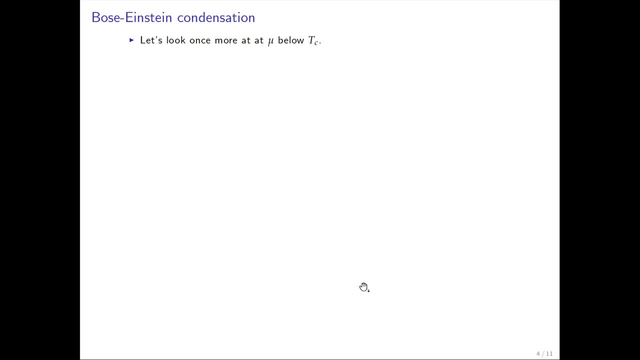 So let's look once more at the chemical potential below Tc, because we discussed this before. So now that we've found the condensate fraction below the critical temperature of this form, we can separate. you know, when we also had separated out the condensate fraction, just. 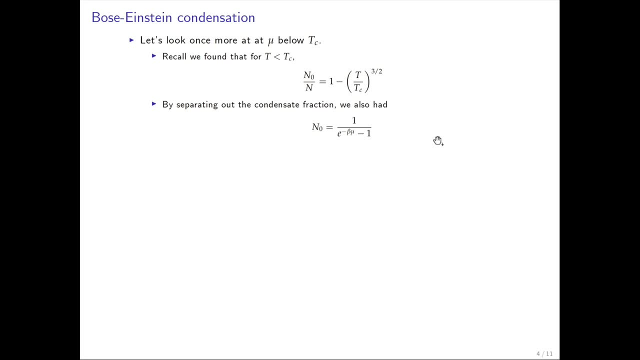 by this Bose-Einstein distribution function. then we can actually solve for the chemical potential And we argued it would have to be close to zero. when it would remain close to zero and we argued before that it would be negative and close to zero and sort of linearly decreasing. 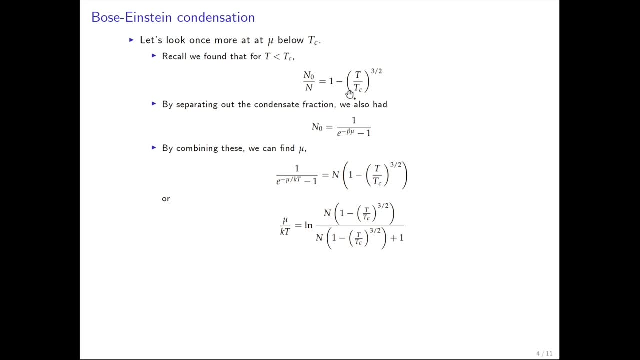 with temperature, at very low temperatures. That's what we argued before. So now that we've done that, we know this, we can, we can turn this around and, of course, solve for the chemical potential and just solving this equation- you get this form here- this: 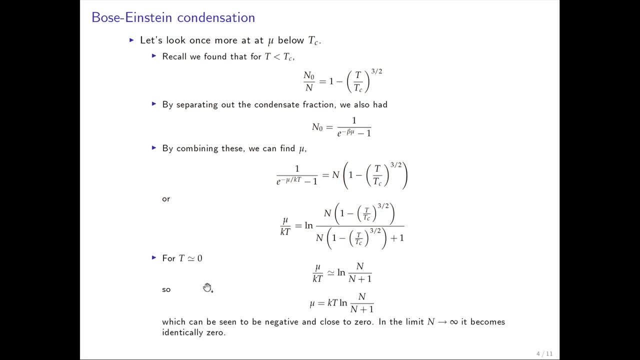 logarithm of this factor here, and you know, for if the temperature is very, very low, we'll approximate this. we'll just take this term is going to be zero very quickly, and so we'll just set that equal to zero as a low temperature approximation. and we have mu over KT, or really Boltzmann's constant KBT is a. 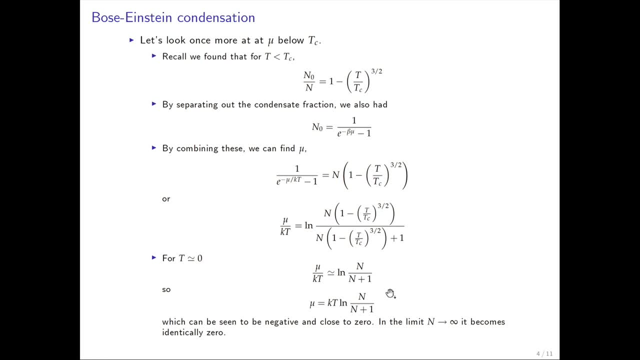 logarithm of logarithm, natural logarithm of n divided by n plus 1. of course that factor is negative because this is n plus 1, is larger than n. so this is smaller than 1. as we said, it's negative and we solve in this limit and we see: 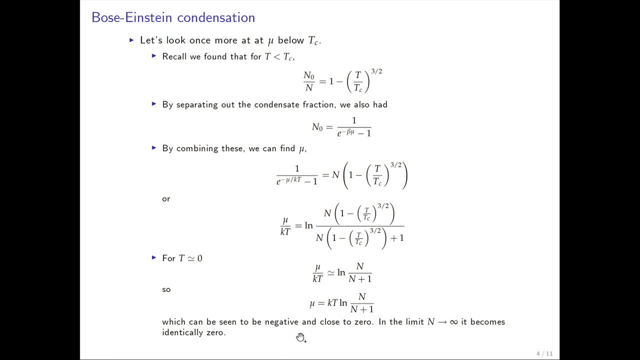 that, as we argued before, it's negative, close to 0, and then the limit that n goes to infinity becomes, you know, really at zero, which is kind of the thermodynamic limit, right, and of course that's you know. well, let's just see how it goes for large n. we just 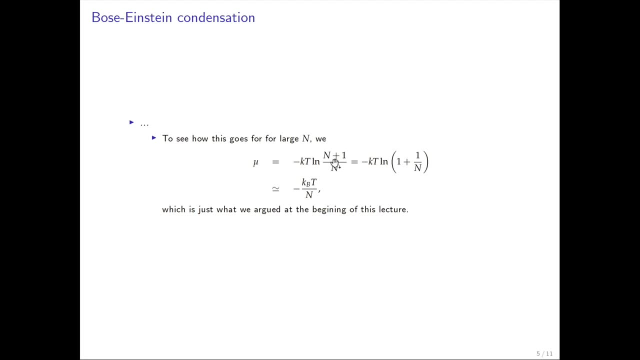 write it that way and if we just rewrite the argument of the logarithm here is 1 plus 1 over n, then of course this term is going to get very, very small. when n goes to infinity and we can approximate the logarithm so logarithm of 1 plus some small factor, is that small factor and and we 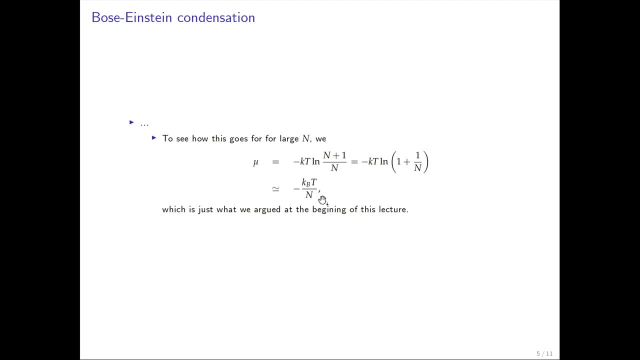 get this dependence for large n, so for large n, the temperature dependence so. so as a thermodynamic limit it's going. it's getting closer by 1 over n and it's also getting closer to 0 linearly with the temperature decreasing. and that's just what we argued at the beginning of this lecture. 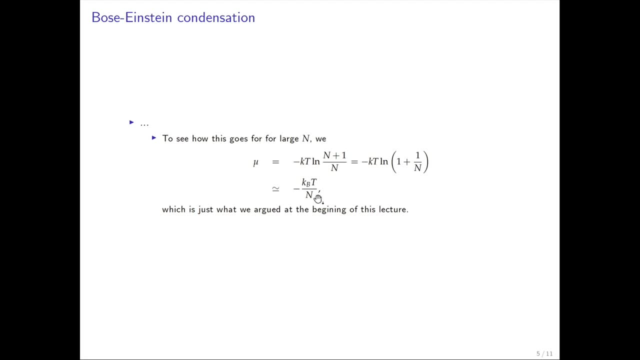 we did some hand-waving arguments and we had, you know, we had an zero here, the number in the ground state, and we said, well, we expected n zero to be approaching n and we sort of used that as the basis of our argument at the beginning. 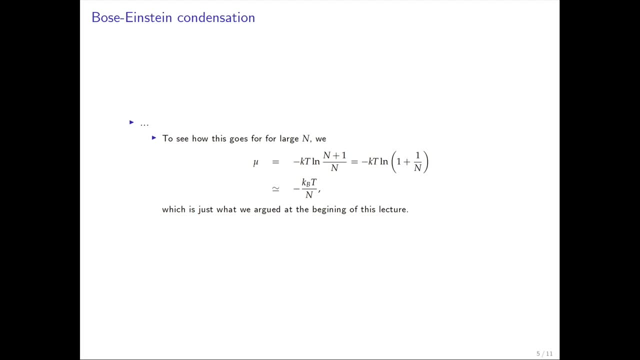 of so actually it was the beginning of lecture 11, actually you have to go back and look at lecture 11 for that, and so it's good to see this, it's good to see this come out of what we found for the actual dependence of the number of particles in the ground state. 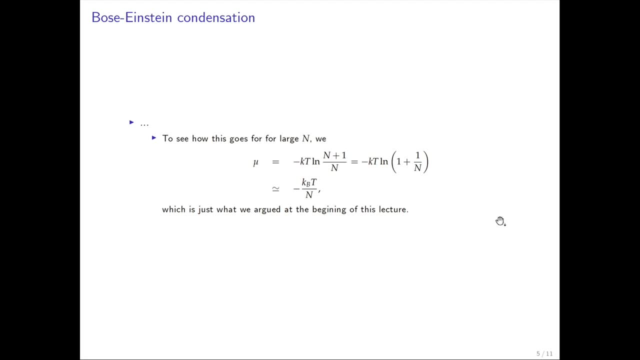 Okay, so another aspect that's interesting to look at regarding Bose-Einstein condensation is this kind of connection to- I kind of call it- the quantum connection, but it's really there's actually lots of connections to quantum physics that we won't explore. this is a rather 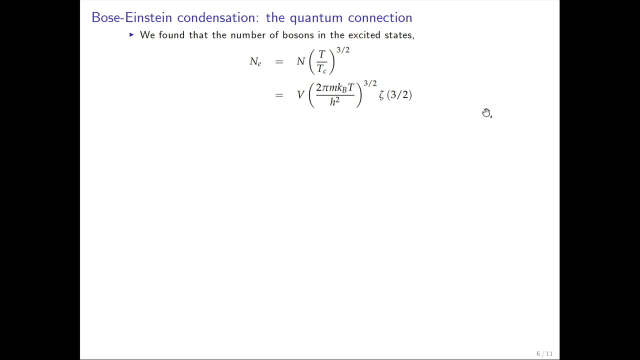 simple one, but it's really worth pointing out. So we found the number of bosons in the excited state Just as I presented in the last a couple of slides ago, as total number of bosons times its factor T over Tc to the three-halves power. 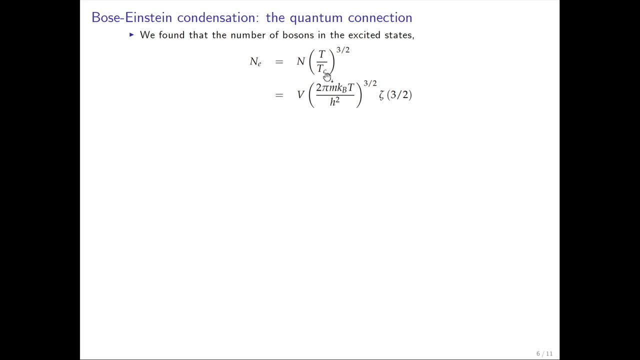 And if we plug in the value of the Tc, we found- we just write it this way- it's proportional to the volume, of course, and to this sort of factor. that's just where we've taken this is basically the inverse of Tc, this factor here. 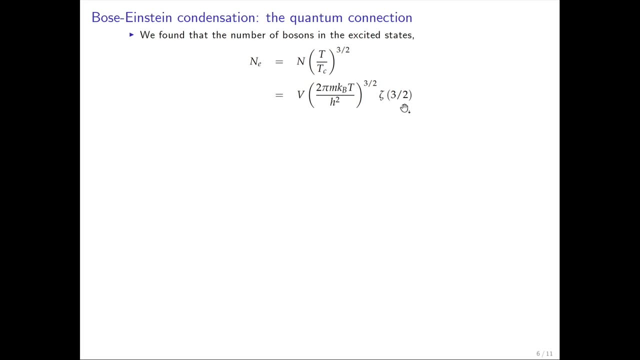 And well, we've pulled out also this constant, This Zeta of three-halves, which was, I think, 2.61 or something. it's just some number. Anyway, now, if you look at this factor, inside this brackets, inside these parentheses here, 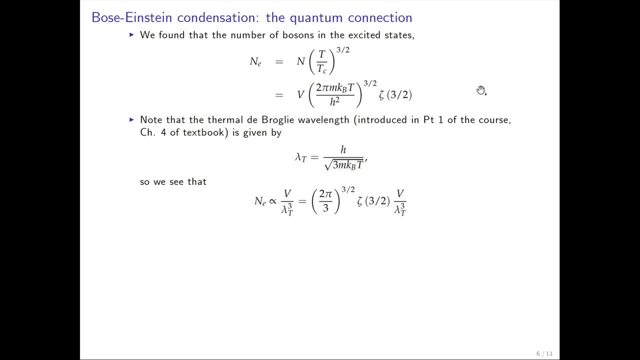 you realize that it you might recognize that it's something like the inverse. it's like the inverse square of the what's called the de Broglie, the thermal de Broglie wavelength, And I think you had that in part one of the course. it's in chapter four of the textbook. 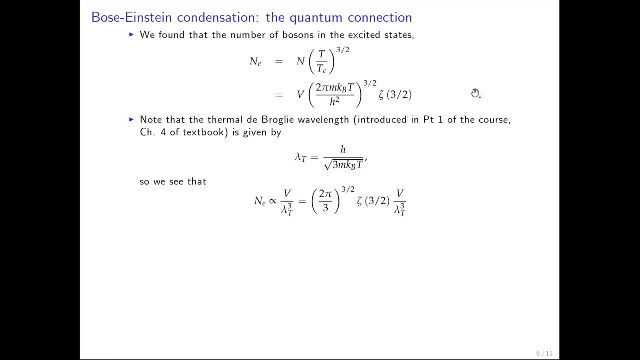 if you want to have a look at that again. But the thermal de Broglie wavelength is just given by Planck's constant H divided by the square root of three times the mass times, kB, T right, And so as T gets really small, this factor is getting really really large and large. 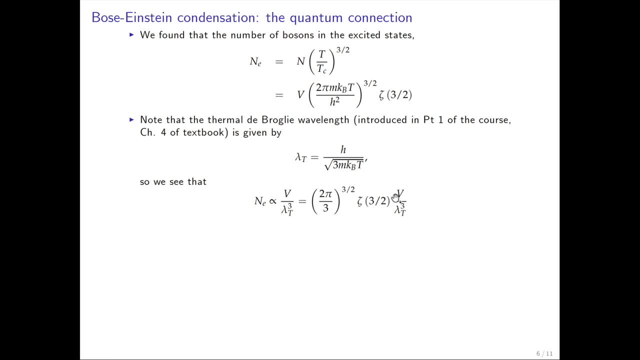 and large. So what we see by recognizing that factor is that the number of particles in the excited state- And remember that above Tc, you know all of essentially all the particles are in excited states because there's very little the factor you know the ground state doesn't. 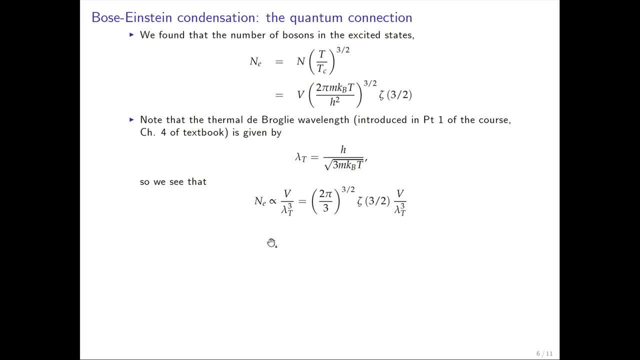 really contribute above Tc, So we can think of this as all the particles basically. Well, we see that the number in the excited state from this is sort of like volume divided by the thermal wavelength of these particles cubed right. So 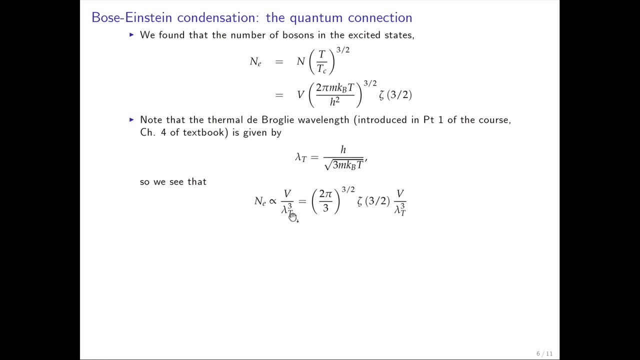 So this is the total volume and this is kind of like the volume that each particle takes up, right, It's a kind of wavelength, these particles, And so of course we expect the number to be proportional to that and you can plug it. 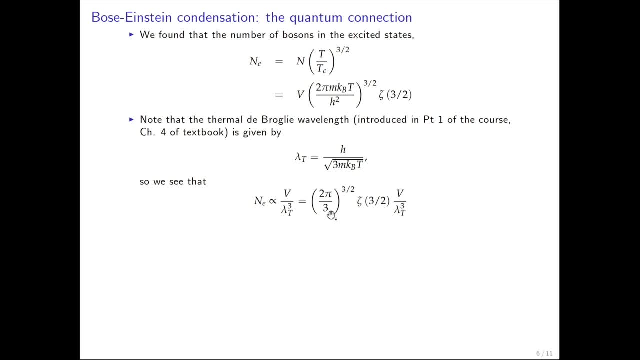 in if you like. You just get these pre-factors here right From this equation by plugging that in So you know, you can imagine kind of what's happening. then That is that you know the. You could say: well, if I know, if I put in the critical temperature, I'd get the value. 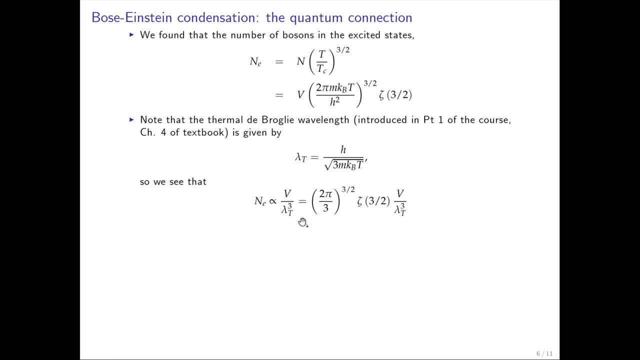 of the de Broglie wavelength at this critical point, and you know what would that correspond to right? And so you know, at low temperatures this becomes this thermal de Broglie wavelength can become very, very large, In fact it. 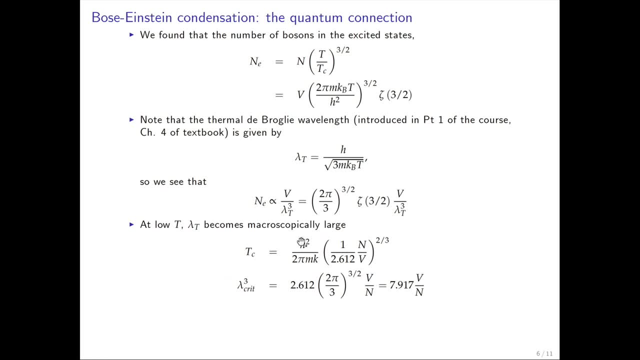 If you, If you, If you put in the low temperatures, it becomes as big as the container that you have the bosons in. But remember, if we took the value for Tc, we could actually plug Tc into this thermal de Broglie wavelength and work out what we get. 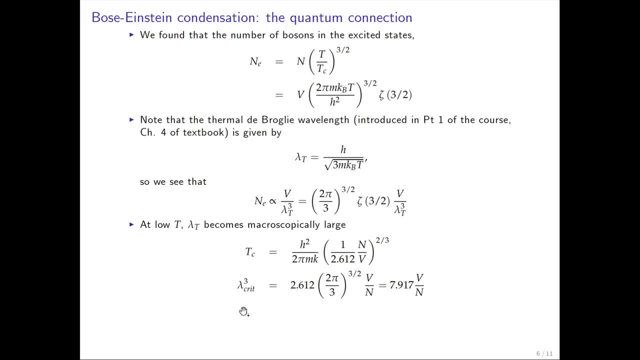 And what you'll find is just this, is that the critical value of Tc means the critical value for this. you know, de Broglie, thermal, de Broglie, wavelength, And it's some, you know Few times, or some several times V over N. This is the volume divided by the number of 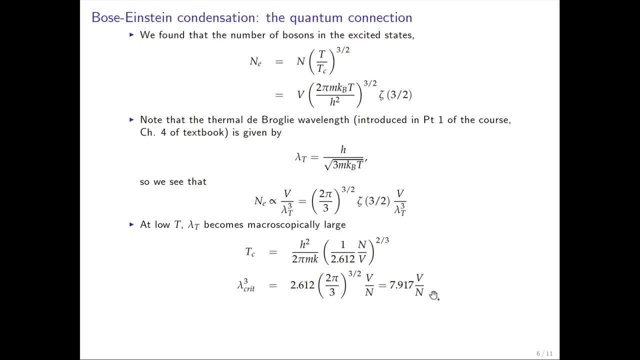 particles. So it's kind of the, the volume per particle, right, Sort of the average volume, that that one of these bosons occupies Times some factor, you know, of eight, right. And so what this is saying is that as you go to low temperature, when the, when, the 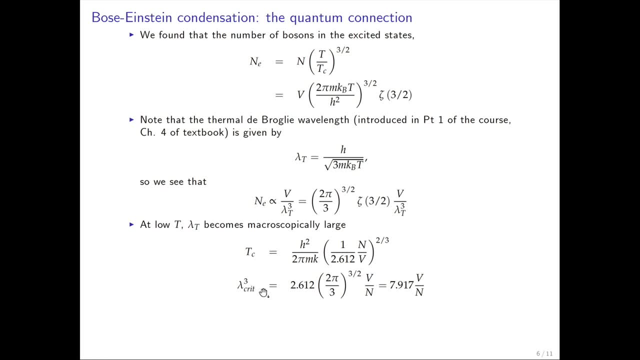 thermal de Broglie wavelength cubed, which is, you know, the volume that the boson occupies, is, You know, several times the the volume per particle. then that's where this transition occurs And what that tells you. it basically tells, roughly speaking, that this transition occurs. 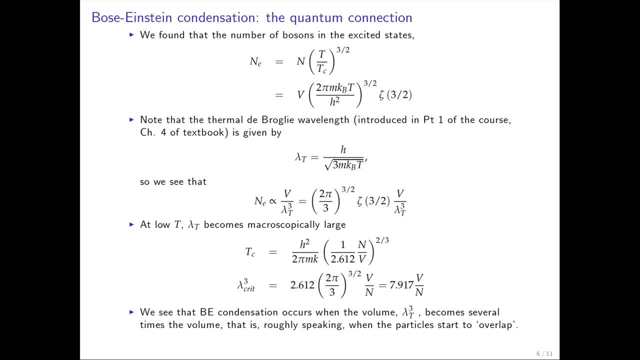 when the particles start to fill each other and start to overlap right. So that's, that's an interesting way then to look at the critical temperature and what's happening Now. there's much more regarding quantum behavior of Bose-Einstein continents. 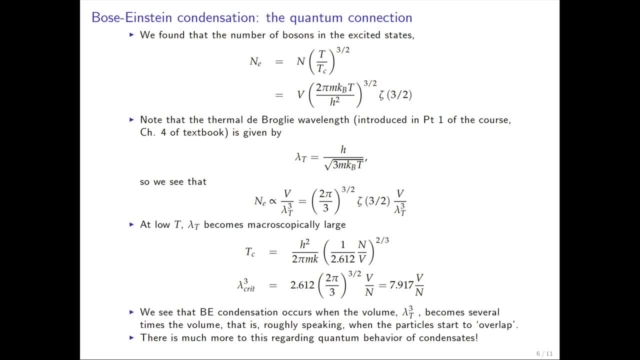 It's a huge, really interesting subject, Because what you find is in this, this ground state, all the particles are in the same state And, in fact, this ground state behaves quantum mechanically in a very coherent, coherent matter. It's like this order parameter, which is the which I mentioned, was like the number of bosons. 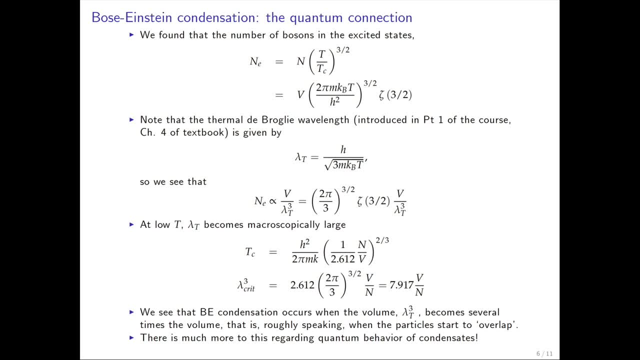 you know It's like the number of bosons in the ground state, It can all be, so be thought of as a, as a kind of a, a macroscopic wave function. that just that describes the, the, you know, all the many particles that are in the ground. 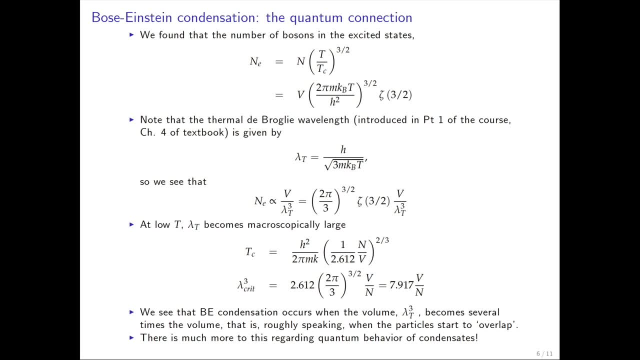 state And they all have sort of in a- in a rough way of speaking, the same wave function And in fact that can have a phase and and that can behave. you have a lot of effects that are based upon quantum coherence of these condensates. 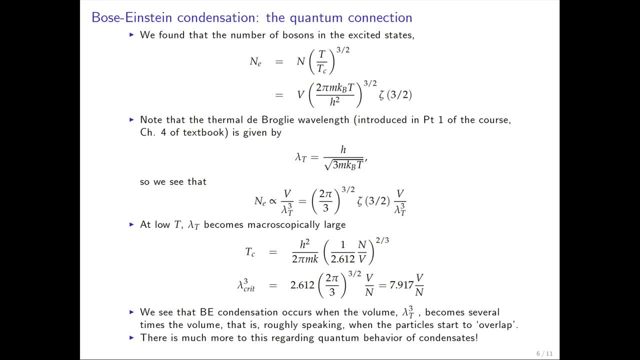 And- and that goes for superconductivity as well- The fact that it, which we'll discuss at the end, superconductivity is- is not really ideal- Bose-Einstein condensation, but it involves something very similar- And the fact that the, the ground state, has a large number of particles described by essentially, 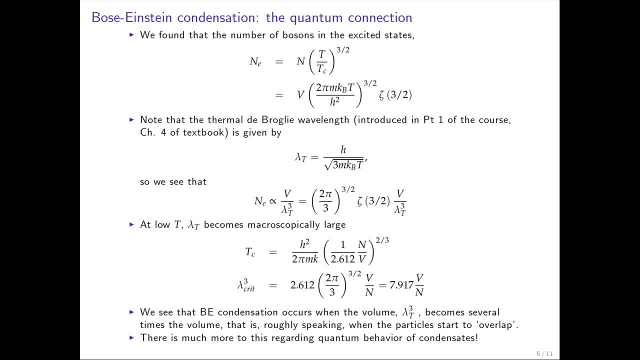 the same wave function leads to some quantum coherent behavior and it's the basis, for example, of superconducting quantum bits. But that's kind of a side story. but I just want to point out to you this way of looking at the transition temperature, the critical temperature and the transition, and, as a way, 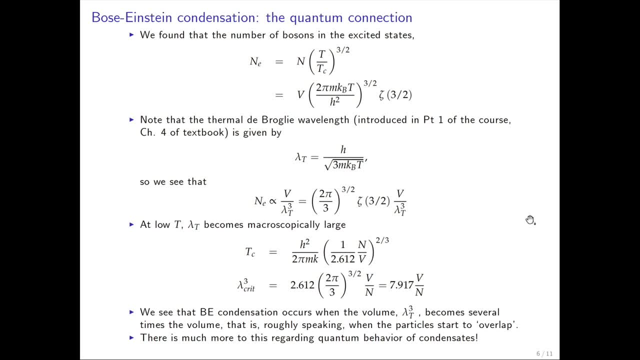 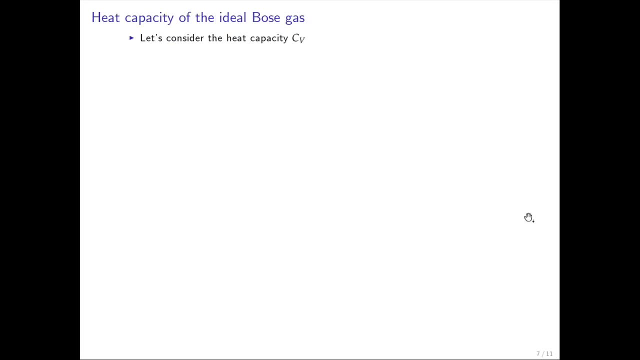 of thinking and point out some other things. All right, So let's continue. then Let's calculate now the heat capacity of the ideal Bose gas at constant volume, So we won't change the volume of the system, and that's called Cv. Okay, 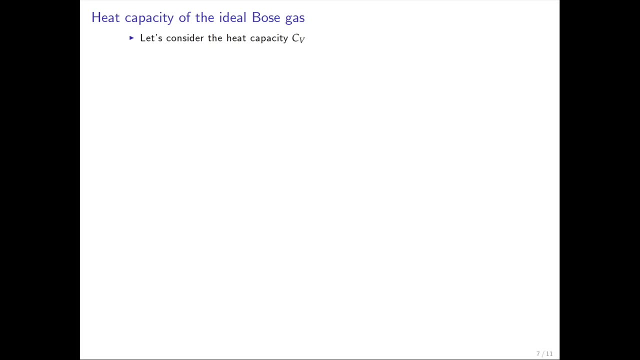 Well, first thing, you, you, you, let's ask yourself, is: how do I get the heat capacity? Well, of course, I have to find the mean energy of the Bose gas, and and then I look at its temperature dependence and I take the derivative. 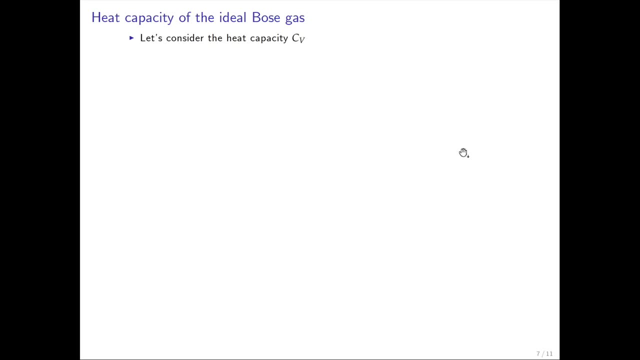 So heat capacity means find the mean energy And then see how its temperature dependence. So but first, before we go run off and calculate things, let's kind of think about it physically from you know kind of conceptual point of view, right? 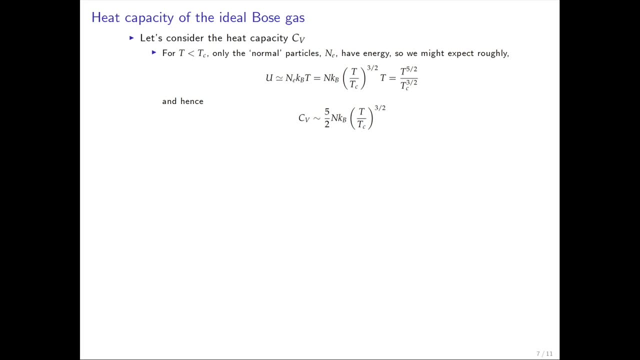 And, and so we saw, we saw that the the below the critical temperature there were, there was a large number of the particles that are in the ground state, which grows as we lower the temperature. And then there's the rest. of them were in, you know, excited states. 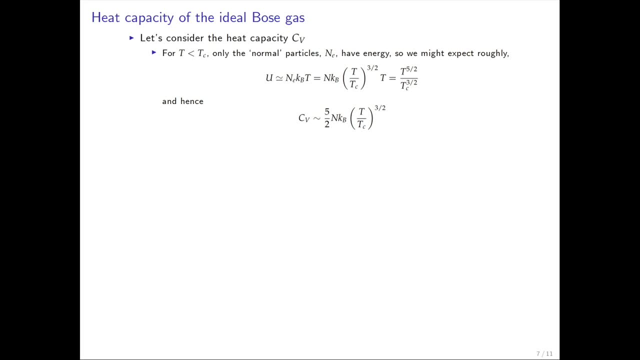 This N, sub E, And, and we can think of these, as you know, normal particles. it turns out They they behave, you know, more or less like usual particles in a box, or or ideal gas particles, let's say right. 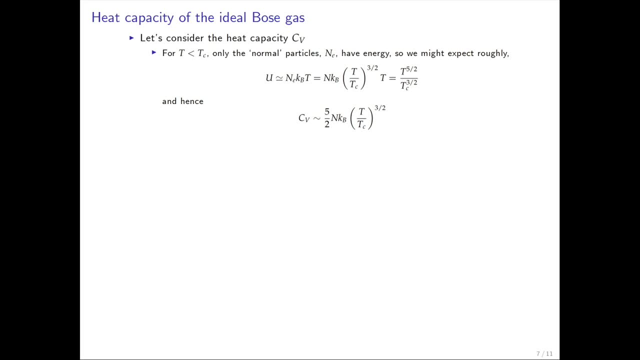 And so you know, for the temperature less than the critical temperature, we we might, you know, argue that you know well, if everything's in the ground state- and we've, we've called that zero energy, of course that's going to contribute zero to this. 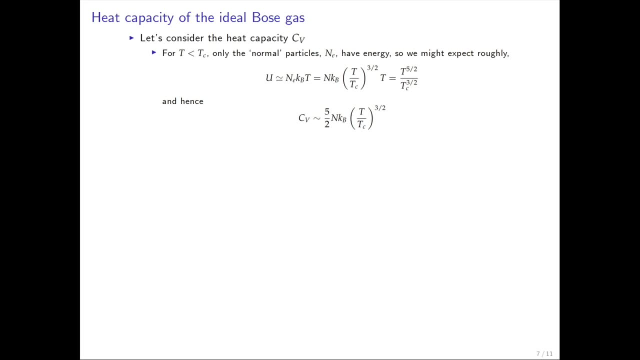 So we might argue that, Well, only the normal particles count, contribute to the mean energy and its temperature dependence, right? So we might expect roughly, of course, that the mean energy is number in the excited states times, you know kVT, right? 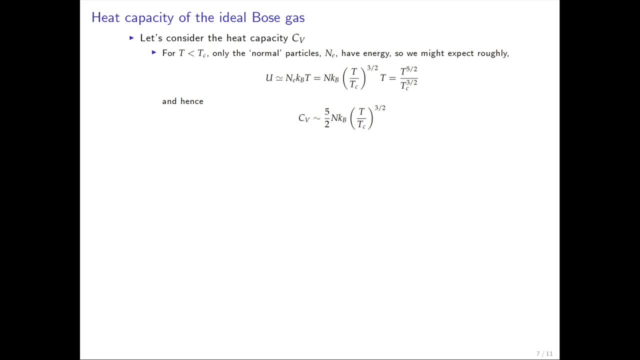 As you, you know, might expect for an ideal gas. let's say: Or this sort of this is sort of an equipartition. If you remember, we discussed the equipartition theorem A few lectures ago, And so we substitute in then this expression for the number in the excited states that 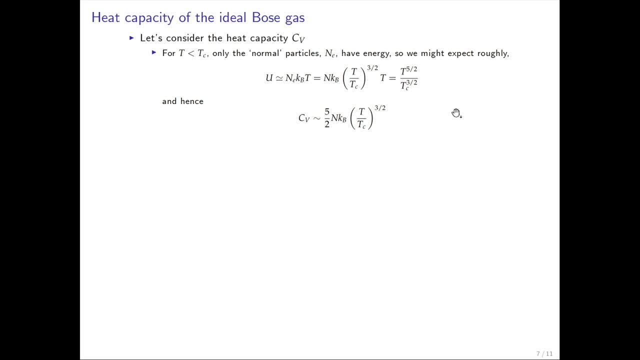 has the n times T over Tc to the three-halves power and and then times T here. So we just substitute this and and then we get, just move the kV over here, and of course we have, you know, something that goes like: well, this is well. actually, I kind of 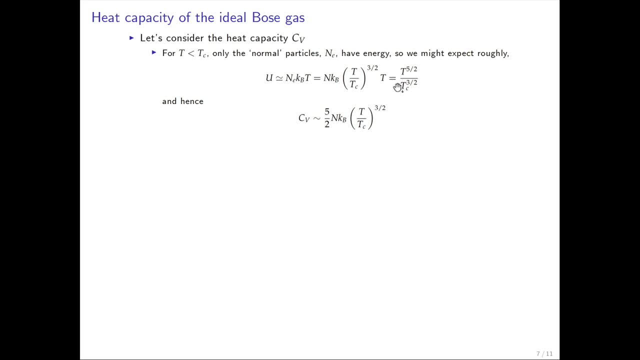 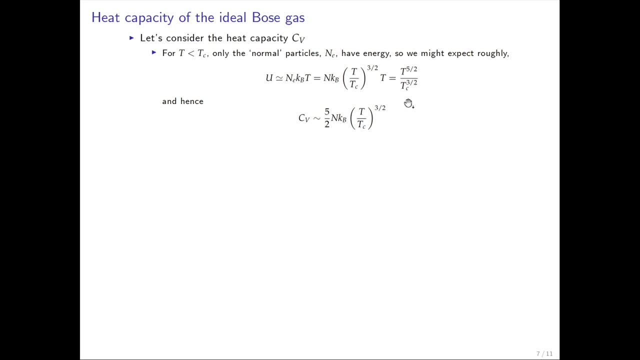 So you can, you can, you can do this, you can do this. And then you, just you know, you can formally use these. you can, you can do this, you can do this. You can, you can, you can do this. 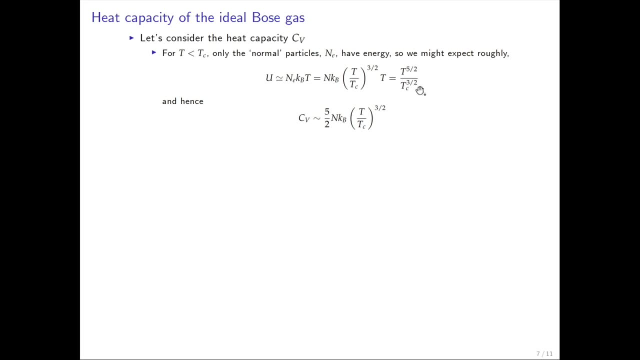 Then you can plants. You can, you can, you can do this, But of course you can do, you can do this, But at the same time the, the, the, the temperature factor is, is the t to the five-halves. 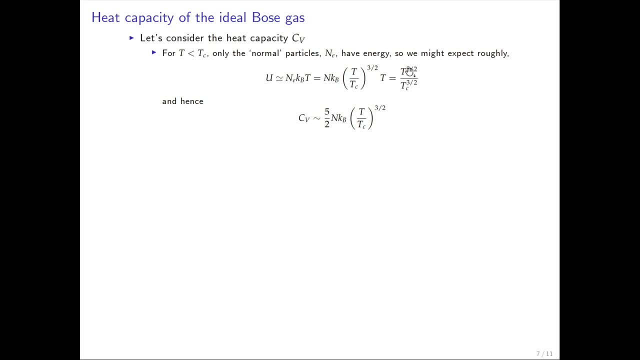 times Tc to the three-half, divided by Tc to the three-halves. So then, if we take the derivative, of course, we bring down a factor of five-halves and thought, well, it's just the normal particles contributing and it's 5 halves in Kb times. 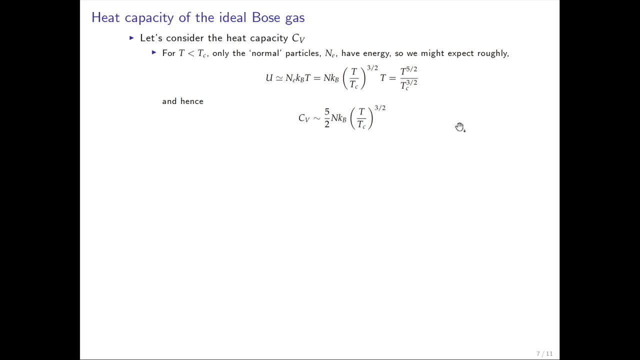 T over Tc to the 3 halves right. And well, you know, that's turns out that that will be a good estimate. We'll actually now we'll calculate that expecting something like this right. Well, of course, to calculate precisely, we have to integrate over the density of states. 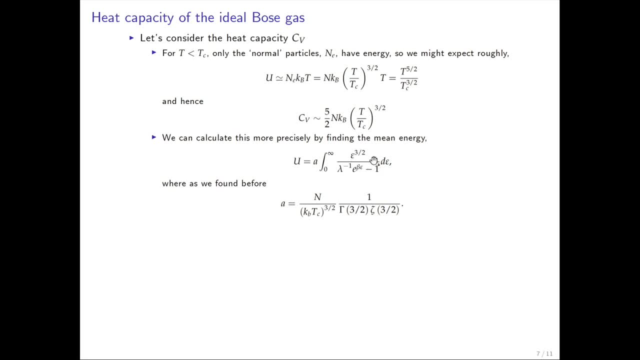 times the energy and find that and integrate from 0 to infinity, as we normally do, And we're going to use this trick again. Remember, we found the density of states in this more convenient factor, which is A times epsilon to the 1 half, and when we find the mean energy. 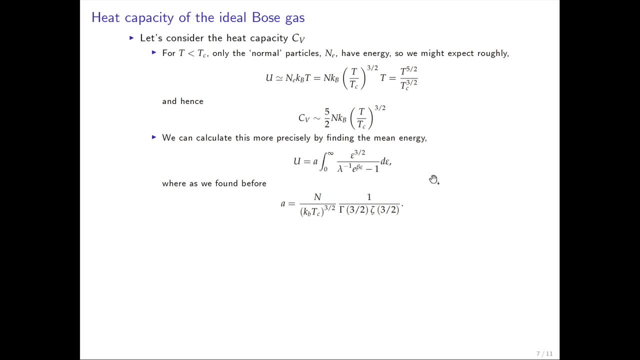 we multiply by another factor of epsilon, so we get epsilon to the 3 halves here. And this constant A we found, you know, by expressing the density of states in Tc rather than this more complicated factor. That's what we found. 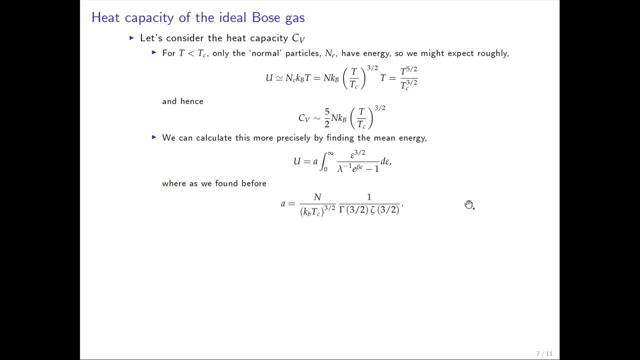 And we used that at the very beginning of this lecture and in lecture 11.. And so let's do that. Well, we still have actually a pretty not so, not so easy to do, let's say integral. Of course, it always can be done on a computer, But let's first, you know, let's to get some. 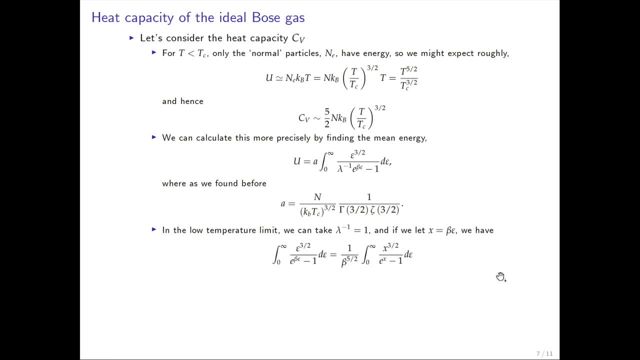 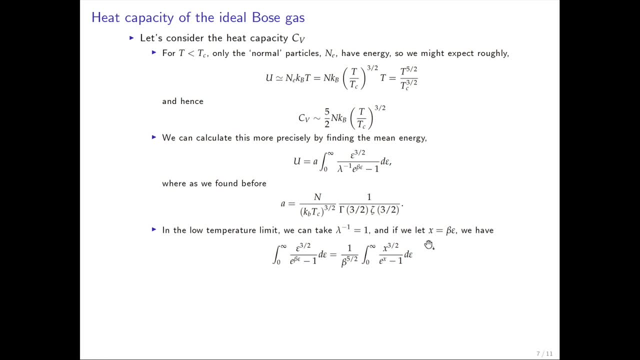 and And and. then we get this integral here. And of course we do the usual change of variables. That brings out beta to the five half here, because we've got, we have x When we have. when we substitute epsilon is x over beta. we get 3 halves from that factor. and 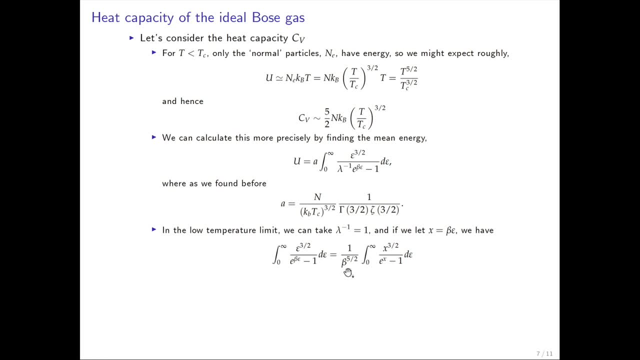 another power 1 from that factor, And that's what this beta to 5 halves. and there we, we, and now we have this integral over x. Oh, I made a little little mistake, So what does that make me thing? Let's start at that Now. let's try to use this. expression in behaviour. is this X over zero? that used to be. And then let's think of distance, is like This I'm going to make, I had a little matrix, This I am going to make. So this Y over one is double, equals Y over two. Now, if you rest it, if you employ this, 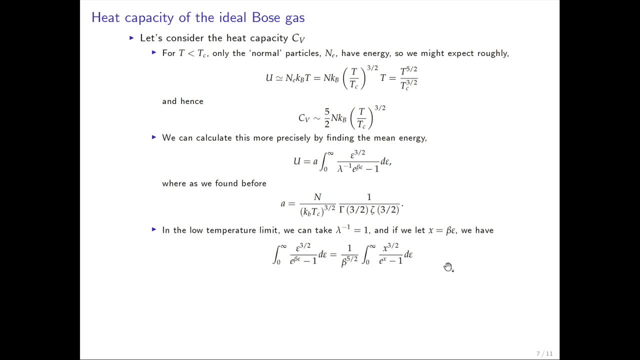 there that that should be an X, of course as well. I'll fix that before I post these notes up to Moodle and we can't quite seen that integral before. but there's actually a result. it's in the textbook and you can find this on the internet and other where other you know people have studied these kind of. 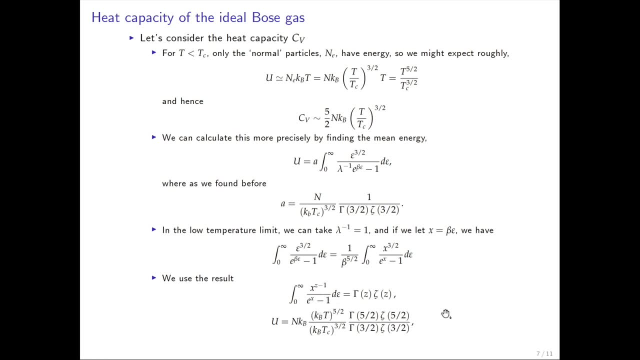 integrals a lot since the early days, and whenever you have an integral- oh I can't believe it, I had this. I didn't catch that from when I was writing these notes up. this, of course, should be an X, but integrals of this form when you have X. 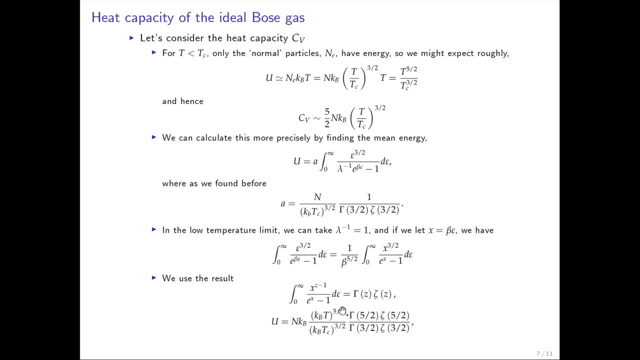 to some power and you express that Z minus 1 e to the X minus 1 over DX, you, you get basically a product of a gamma function of Z and the Zeta function of Z, and and of course, these are just numbers. right, these are just numbers, and 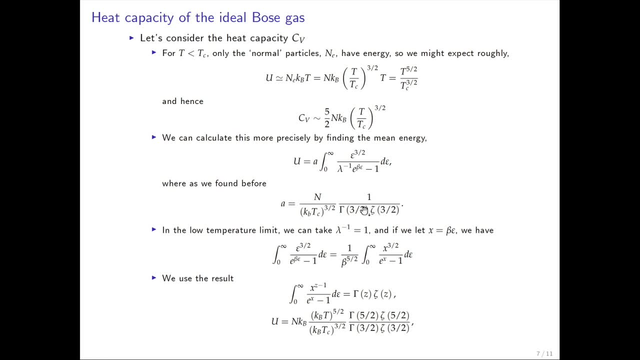 remember we had this a here that we found from the number constraint and, and, and and. now, if we complete this integral, we get something that's fairly easy with. in fact, it's very much like what we guessed up here. it's just that we have different factors out here and these are- these are just numbers and can. 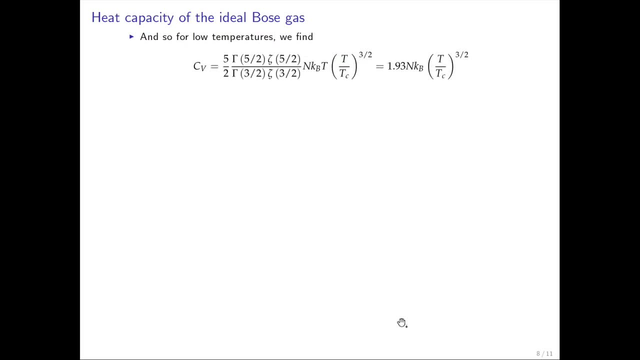 be evaluated, by the way. so do I have those numbers there? I don't have these numbers, but you can look now. I think there's actually a table we've already looked up the values for here and like this was, I think, gamma 3 of us possibly. 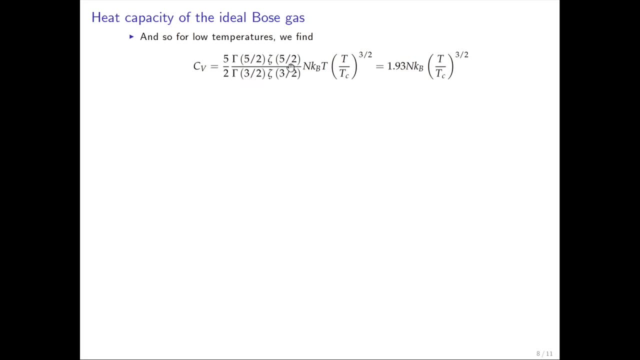 square root of pi over 2, or was a pi square root 2? they're, they're just numbers and if I collapse all these numbers in the 5 half together, I get you know 1.93 to 3, significant figures. there's more if you want, but because it's. 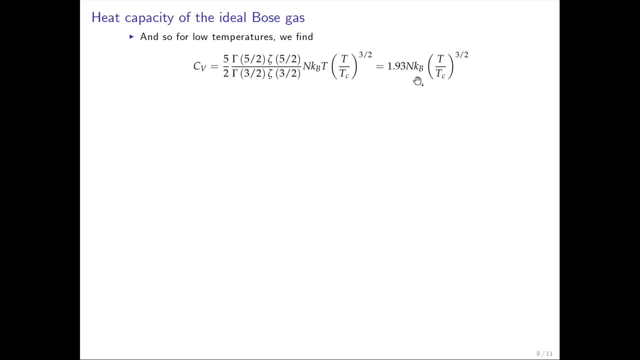 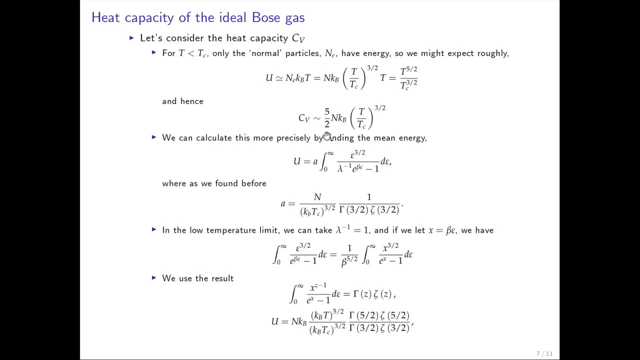 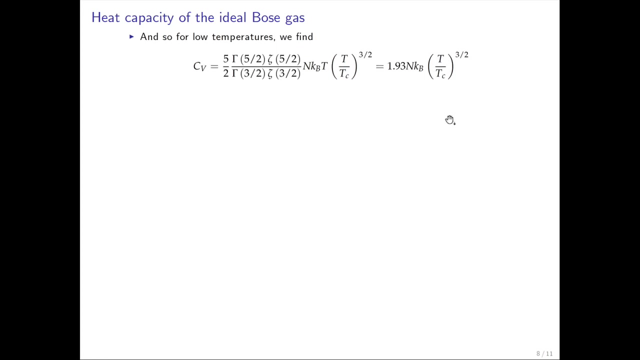 interact, because these are irrational numbers. and what do we get? yeah, about 2 in K, B times this factor. and what did we have before? for we had 5 halves. so so this was pretty close. you know well, that's for low temperatures and that's for low. 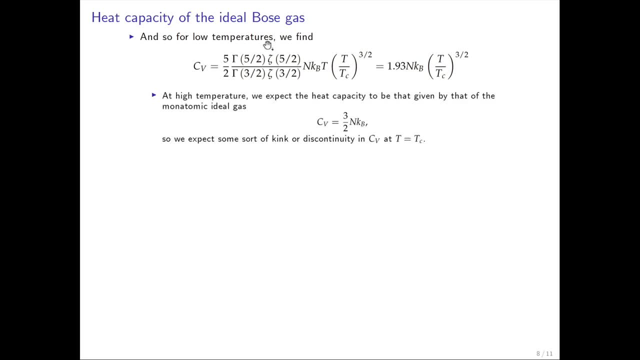 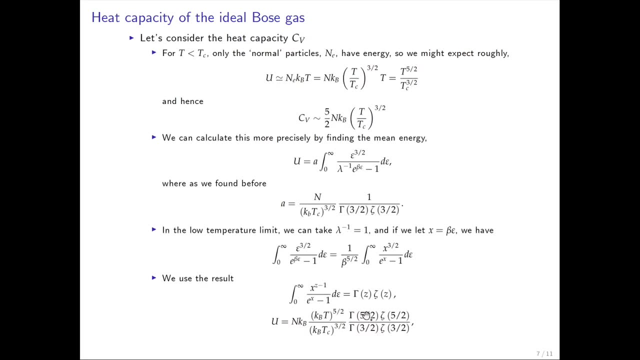 temperatures. now, what do we mean by low temperatures? well, we'll come back to that because we let's, we had, we had to make this approximation to do to actually get this integral in an easy form. at low temperatures we don't mean just T below TC, by the way. we need, we need, we know that, we mean you know when. 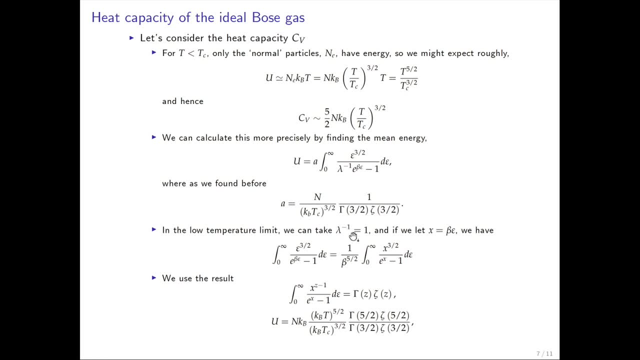 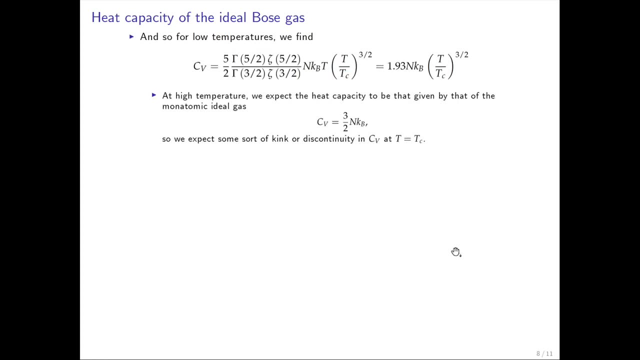 X is small. well, you can see what we need. we need, you know, beta over epsilon to be small, but anyway, we'll come back to that. well, what about high temperature? what do we expect it, you know, at high temperatures above the transition and where the thing is behaving essentially classic, classically, well, classically of. 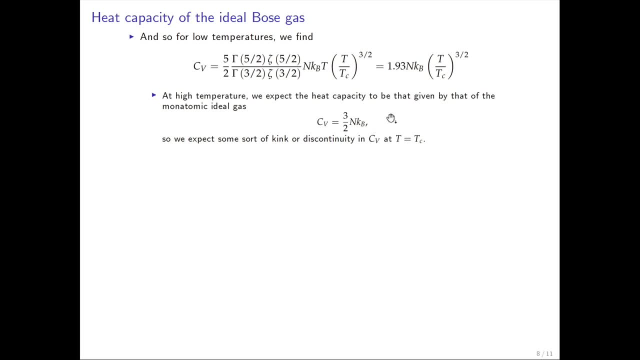 course we would have three halves in K B. right, that's what we get, remember if our arguments about the echo partition- that at large temperatures Bose and Fermi, Bose-Einstein and Fermi gases behave like ideal gases. So that's something that is increasing with temperature. 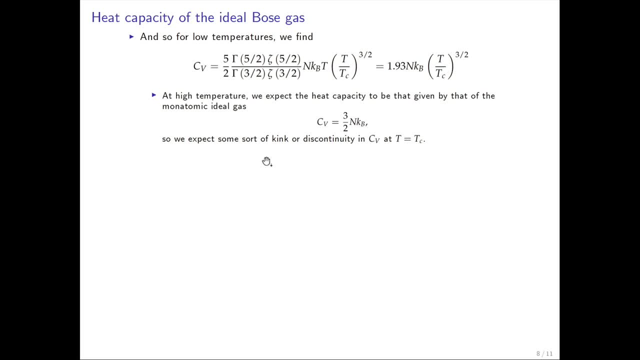 and that's something that's flat with temperature. So, on the basis of this argument, we would expect some sort of kink or discontinuity, or maybe both, at this critical temperature. But we have to be careful, as I said, because this approximation of the inverse fugacity. 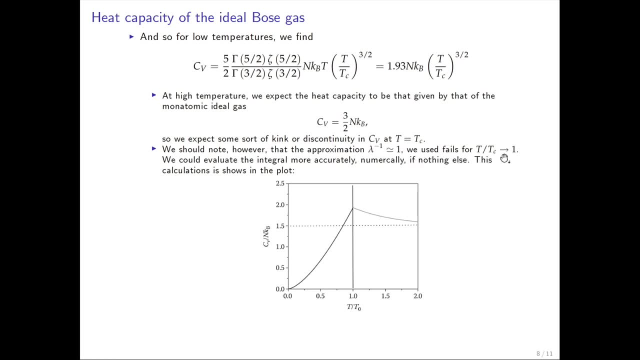 being 1, it actually fails when the temperature T over Tc goes to 1.. It's not quite good for that, But it's no problem. We just have to evaluate this integral. you know this integral here more precisely. You can always do that numerically. 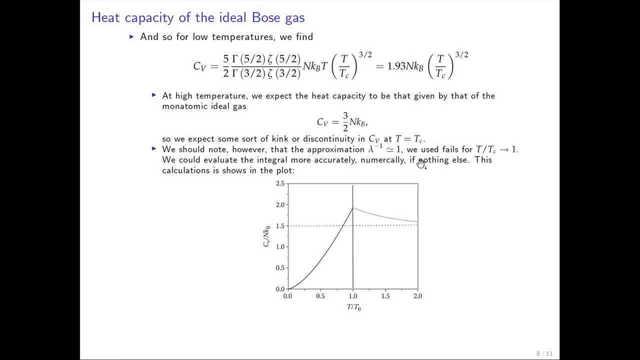 There's always other approximations you can use as well. by the way, There's a sort of systematic approximation Like the Sommerfeld expansion we did in Fermilans. So it's no big deal really, But you get pretty much the general behavior. 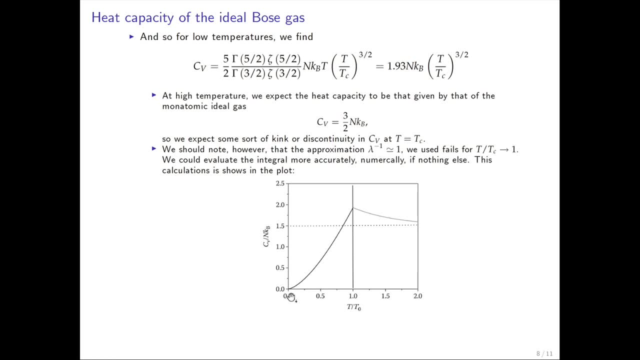 What is found is shown in this plot. At low temperatures you do have this increasing heat capacity, that sort of increases like that, And then at the critical temperature. this is from the book. he uses T0, and I'm using Tc. 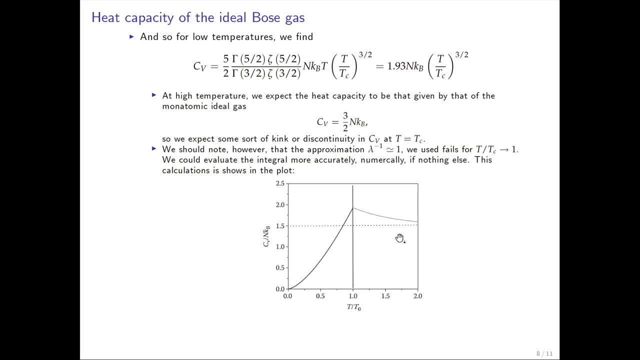 But this is at 1.. And then, instead of going it's flat, it actually just falls off slowly this way as well. But you can see it approaches the classical limit here as we go to high temperature. right, this 3 halves here. 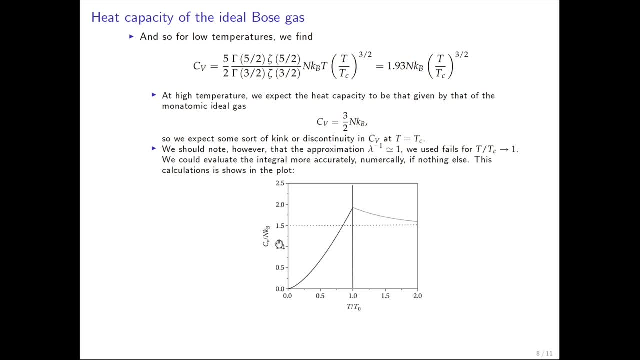 So, yeah, this is the usual way we like to plot the heat capacity and we divide it by N, number of parts and KD, So it's dimensionless. And yeah, so that you know that's what the heat capacity does. 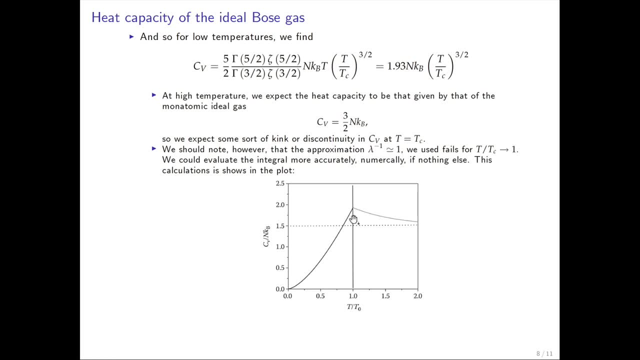 And we notice that it does have a sort of cusp or a kink. No discontinuity though, but it has a kink here And, as we mentioned, with the order parameter or the condensate fraction at low temperatures, this kink is generally what happens at a second order. 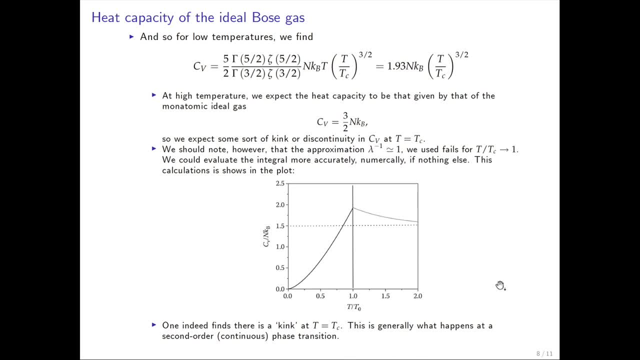 or continuous phase transition, that you get a peak in the heat capacity. In fact you've seen- you may have seen that also in sort of magnetic models for the magnetization, when the specific heat also has a kind of peak at critical temperature In magnetization usually you get a peak. 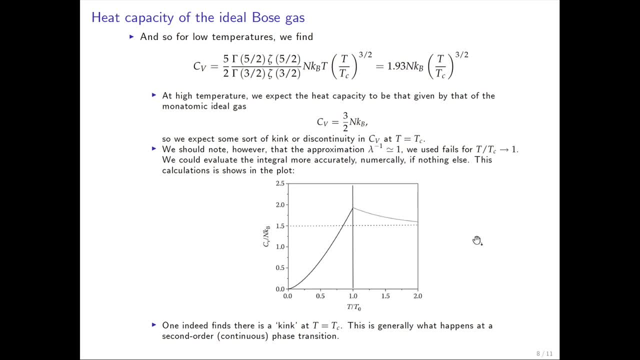 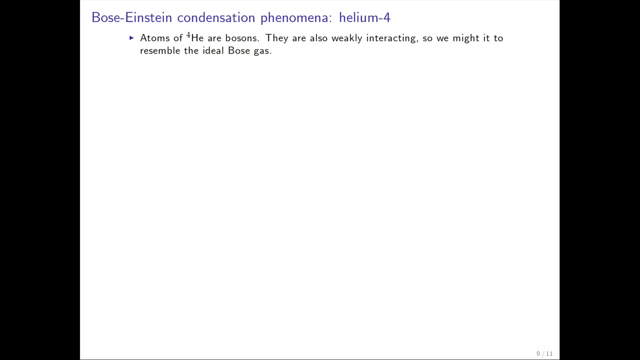 and a discontinuity as well. So, but it's typical, for this is very typical for the specific heat or other sort of what we call response functions at second order phase transitions. Okay, Well, you know, this is a really interesting phenomena. 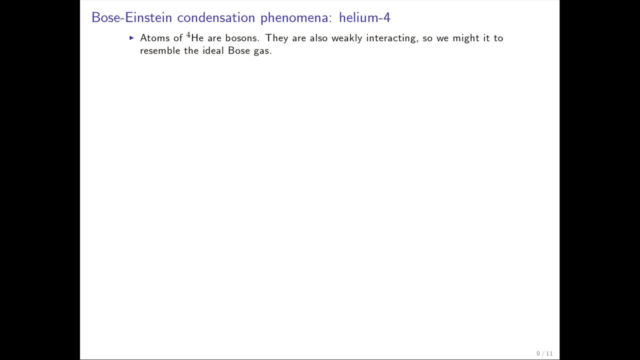 And in fact it was predicted a very, very long time ago in the early part of the 20th century that there's this idea of Bose-Johnson condensation, And it took a very long time for people to well, for people to really experimentally realize this. 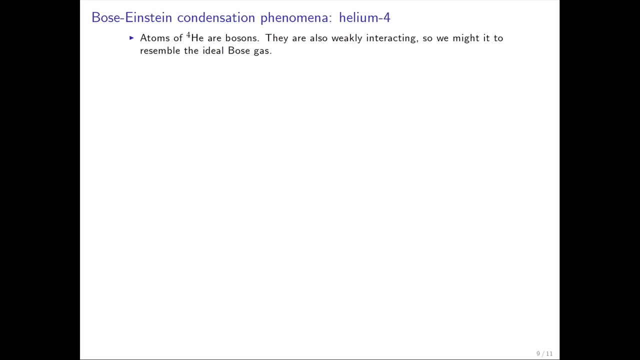 And even though, that being said, it was what we know as superfluidity was discovered in liquid helium, which we'll discuss here on this slide and the next one, And it, you know, was suspected because of the properties of superfluid helium at low temperature. 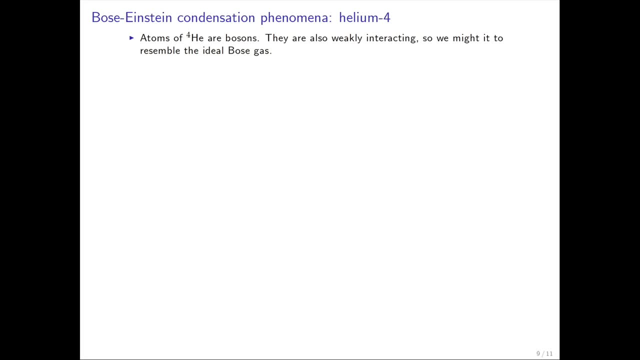 And you know it was. you know the fact that there's no viscosity and other things that probably maybe it was some related to Bose-Johnson condensation, which it is, But it took a while, kind of, to work that out. 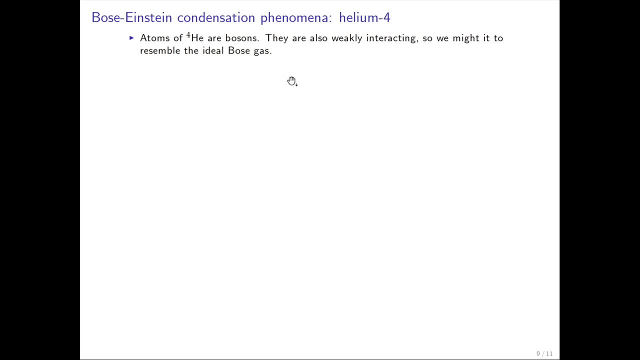 We'll come back to other types of condensation phenomena that are analogous or contain some of the same physics as Bose-Johnson condensation. Experimentally, though, it's hard to reach an ideal Bose gas Because, you know, particles interact. 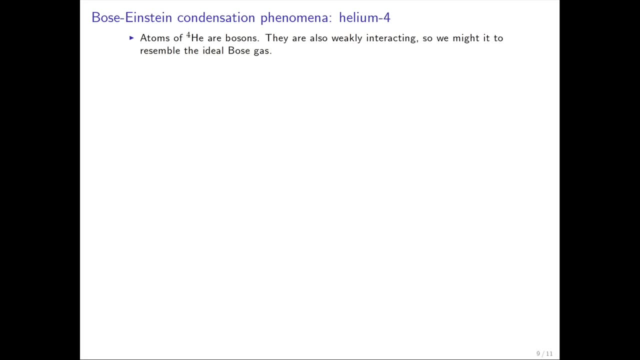 And in the ideal Bose gas, you know we assume no interaction And you can imagine if you have something where all the particles are getting down into the same state, the ground state, at zero temperature. ignoring the interactions becomes a bit problematical. 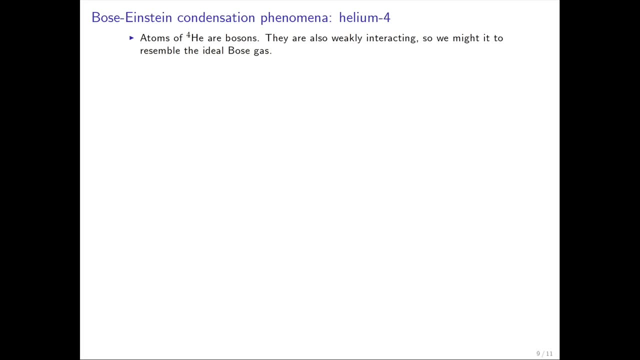 let's say So anyway. well, atoms of 4, HE, and so of course you find, with helium there are two isotopes There's. we call them helium-3 and helium-4.. Helium-4 is the nuclei, are two protons and two neutrons. 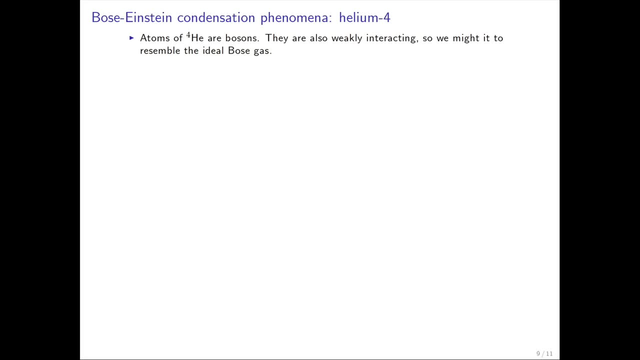 So it's an even number of fermions, And so helium-4 is a boson, And of course it has an even number of electrons too, if you want to consider molecular, which is important here. So they're bosons. 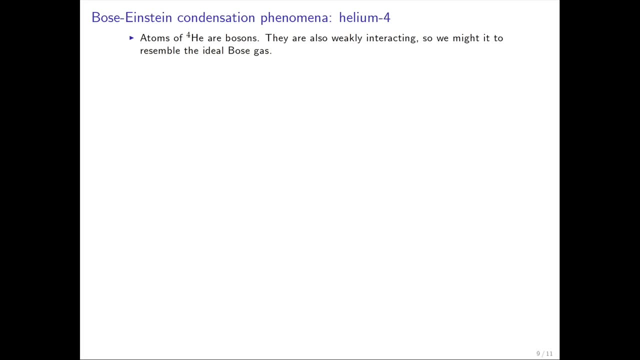 And they're, you know, they're quite you know, they're actually very, very weakly interacting, which is why helium is so important. It has such a low boiling point, And so we think we might, you know, we might expect it. 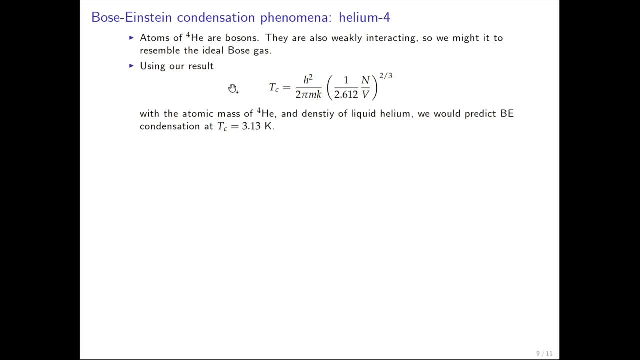 I should say expect it to resemble an ideal bolus gas. And if we used our result for TC, we predicted the critical temperature and it depended on the Planck constant squared, the mass of the particle, Boltzmann's constant, here just this number factor. 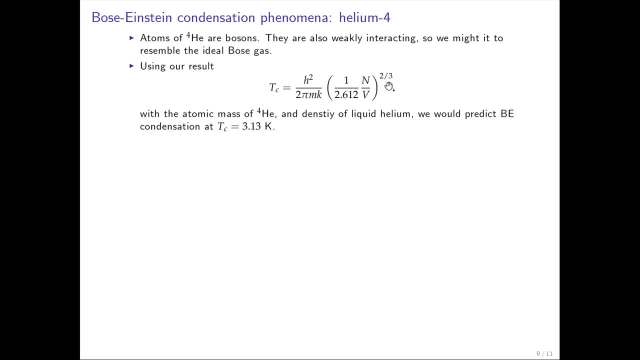 and, more importantly, the density, the number. density to two-thirds power. If we use that, we know, we know the atomic mass of helium-4, and we know the density of liquid helium, we could predict the bolus-Einstein condensation. 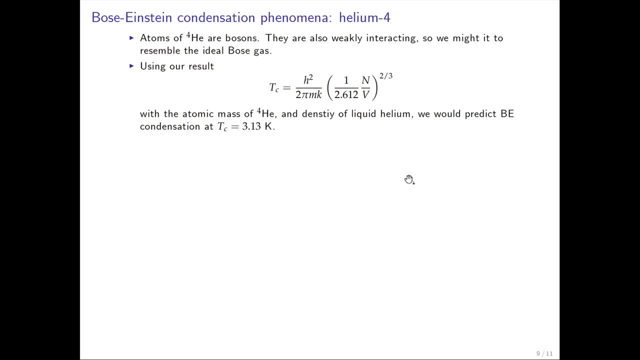 temperature and we'd get 3.13 Kelvin. Well, liquid superfluid helium- sorry, liquid helium-4- does exhibit a superfluid transition, and it actually occurs at 2.17 Kelvin, a bit lower than this, And so it's called the lambda transition. 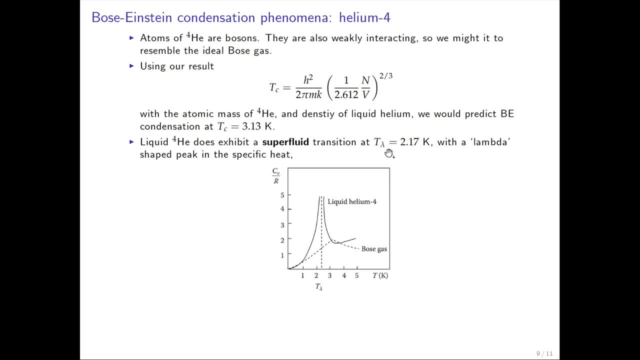 And the reason why you hear it called the lambda transition and why it's usually the critical temperature is denoted T sub lambda is because if you look at the specific heat, in that case the specific heat of liquid helium-4 has this: 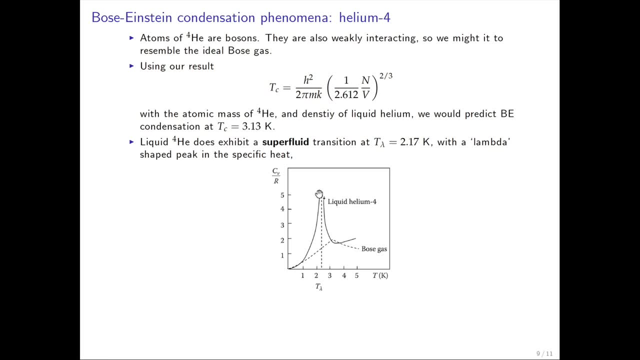 behavior. it's really sharp peak and it actually has a bit of a discontinuity up here and it looks like the Greek letter lambda. So it's a little bit like the Greek letter lambda, So that's how it got the name: the lambda transition. 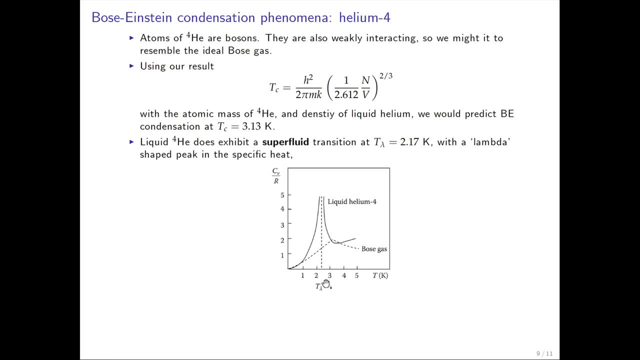 And so on this plot. you see, here's the lambda transition for superfluid helium, transition at 2.2 Kelvin, and this is the heat capacity. that's what it looks like for liquid helium and this is what we calculated for the bolus gas and this is where they go, you know. 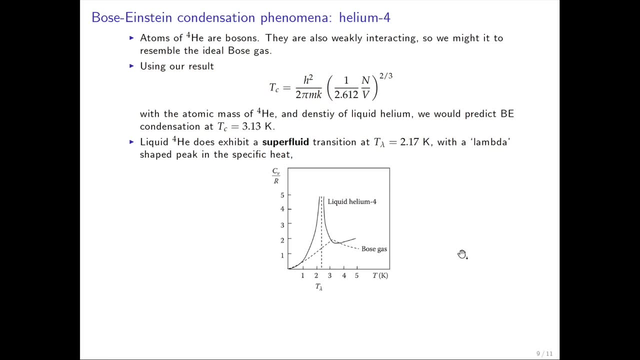 if we would just predict it. So there's obviously, you know, it kind of looks like it's bolus-Einstein condensation, which in a way it is. it's just more complicated and it gives a different heat capacity. 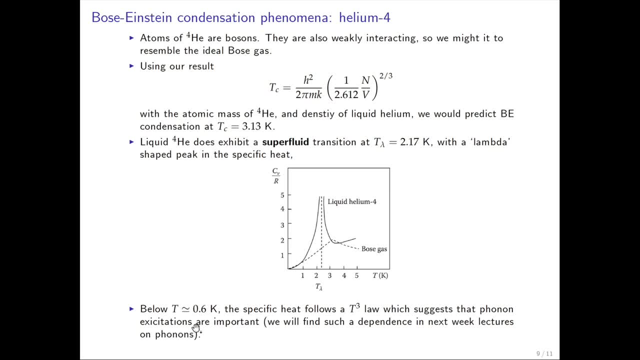 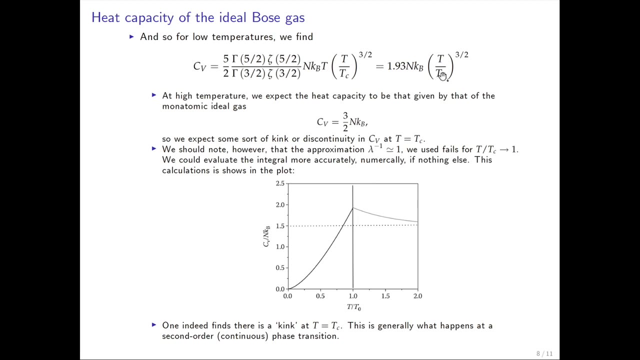 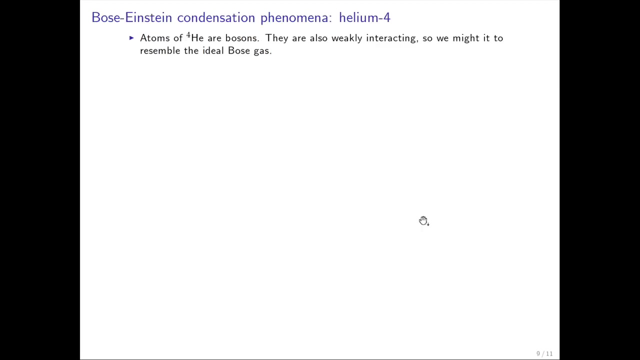 And the other key observation was actually the behavior of the heat capacity down in here. right, And you know we predicted so if you go and look back here. we predicted the heat capacity to go like T over TC or at low temperatures go like T to the 3 halves power. 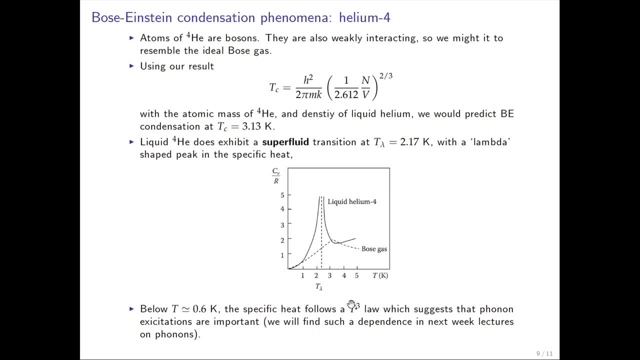 Right, And here it goes like down here, what's found experimentally. it's much sharper, it goes like T to the cubed and that suggests that phonons are important. Well, basically, in fact, next week when we study phonons, 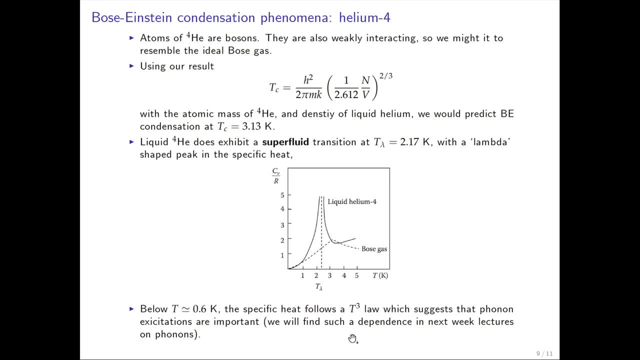 and we study the heat capacity of solids due to phonons, we'll see. we'll derive this T to the 3, dependence and specificity. So what does that tell you? I mean, I guess researchers in the early days realized that. 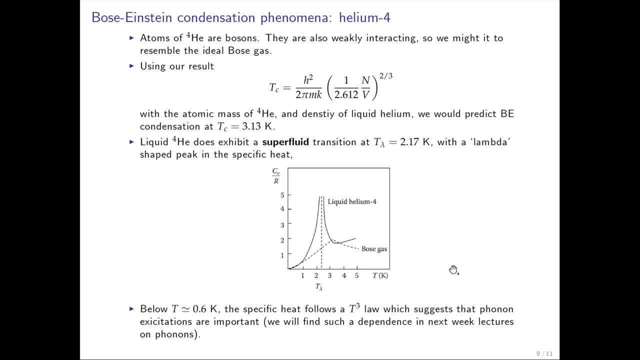 you know that helium-4 was not an ideal bolus-Einstein condensate And even though there's a lot of similarities and it's due to the interactions and phonons which arise, because, you know, atoms attract and repel each other and like to sit. 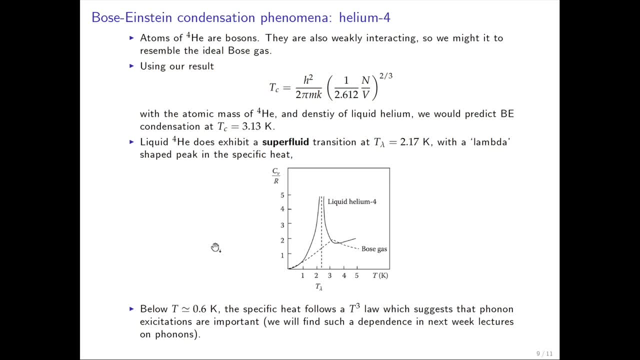 at a certain distance. you know, basically, the Lennard-Jones potential, If you heard that- for something like helium is important and has a lot to determine the properties of this. Nonetheless, it is a type of, if you can think of it. 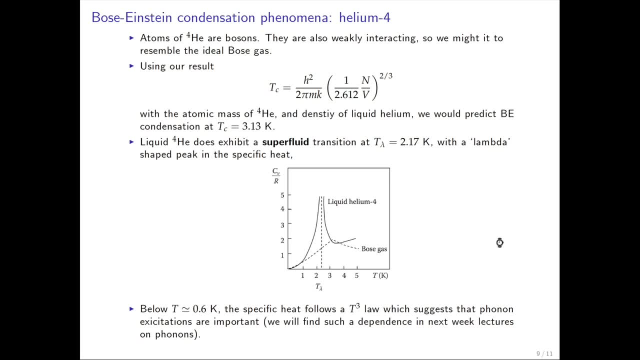 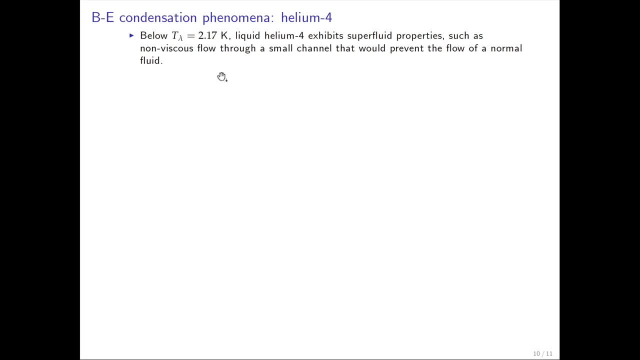 it is a condensation of bosons. Okay, So below this lambda transition at 2.17 Kelvin, this liquid helium-4 exhibits superfluid properties And we mentioned that in principle a Bose-Einstein or not in principle that a Bose-Einstein condensation. 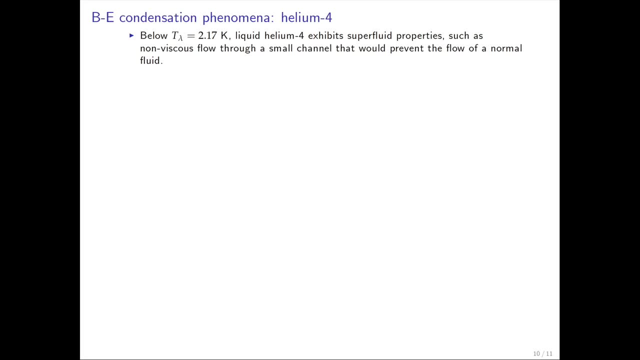 that the ground state, as the condensate didn't, was non-viscous right. So superfluid helium-4 does exhibit that In particular, you have flow through a small channel that you know non-viscous flow. that wouldn't be. 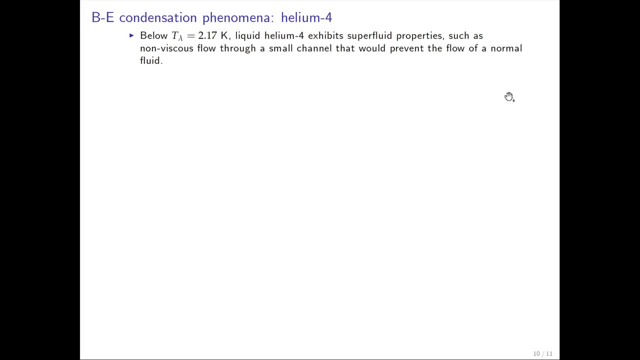 that would actually prevent the flow of a normal fluid. So you make a poor. you know small enough that a normal liquid would, because of viscosity, wouldn't be able to go through it. Then superfluid helium has this property of what we call a superfluid. 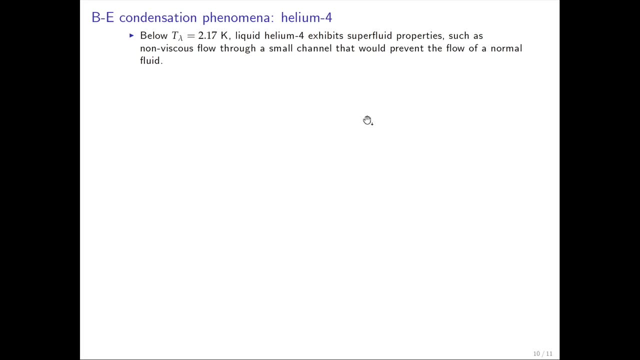 In fact, this is a very annoying property of a superfluid helium if you use it for low temperature experiments And, for example, in my lab or a lot of the labs here, and you know these days a lot of the low temperature. 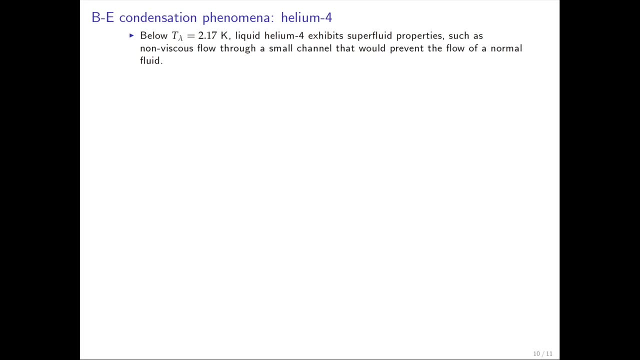 you know, apparatus we buy is made pretty good And you know, in the old days. or if you have a piece of low temperature equipment that uses liquid helium and you go down to very, very low temperature and, for example, 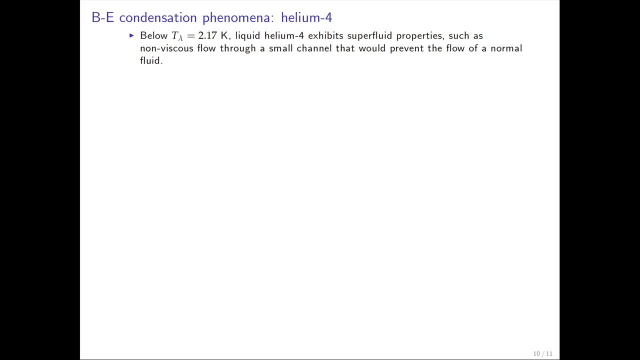 it's old. it's very annoying because sometimes you have a leak because you have some small crack somewhere And when the liquid helium becomes superfluid it will leak right through it And it's very hard to diagnose because you know. 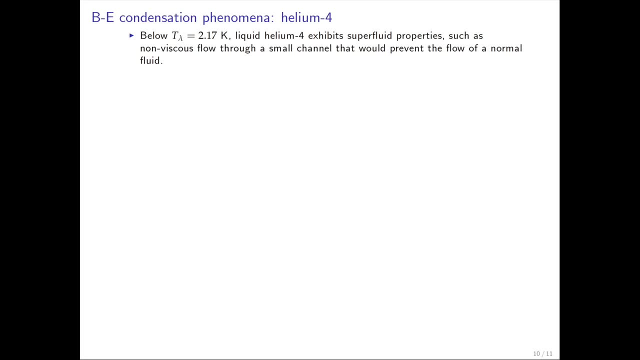 you have to warm up to look for things. Then you know you have to. you know you have to, you know you're not going to see this And then so you have to cool everything down again And you get this super leak. 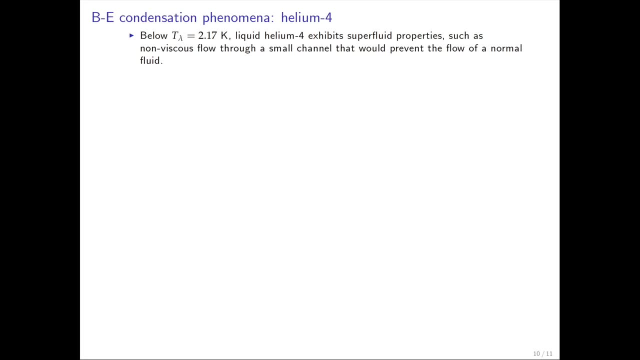 And you know I could tell you stories about people that work for months trying to find super leaks in their equipment, Anyway, but it also has. you know, these properties are also extremely amazing as well, And we'll get to that. 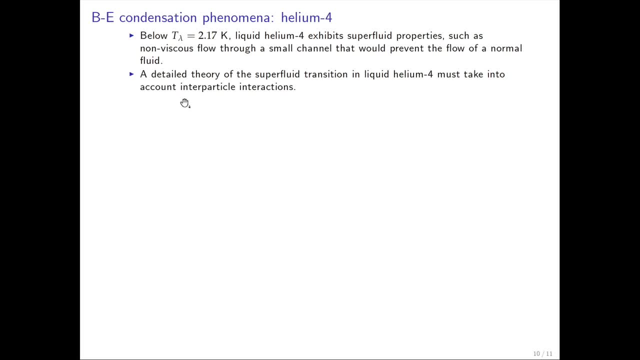 That's only one of them. So the message is, though- and we're not certainly not going to cover this in this course, but a detailed theory of superfluid transition in liquid helium 4 has to take effect, And we'll get into account these inter-particle interactions. 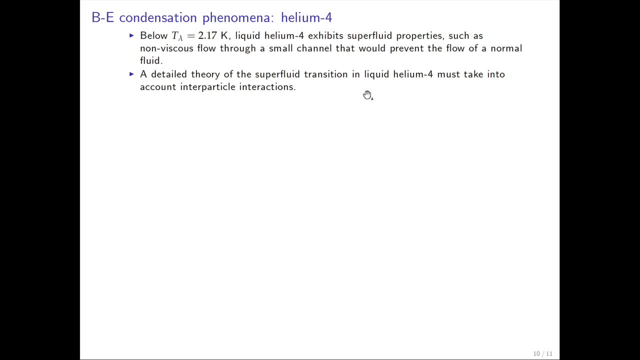 And it took some time to actually develop this theory. This was still being worked on. well, a lot maybe in the last century, but it's still the details. people still work a lot on certain aspects of superfluid helium 4.. 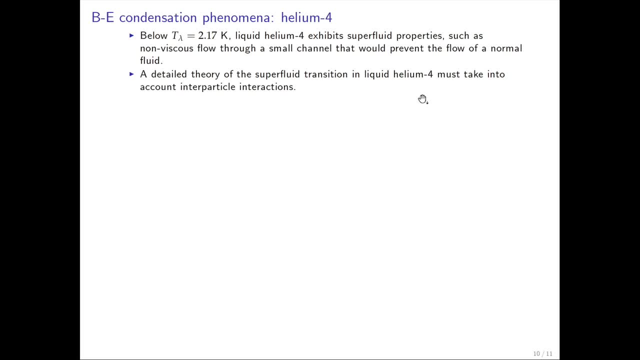 And there's actually been a bit of a renaissance in it now that people can make nanostructures and make superfluid helium. So you know, we don't need to worry about that. It's just going to be a guy doing it. 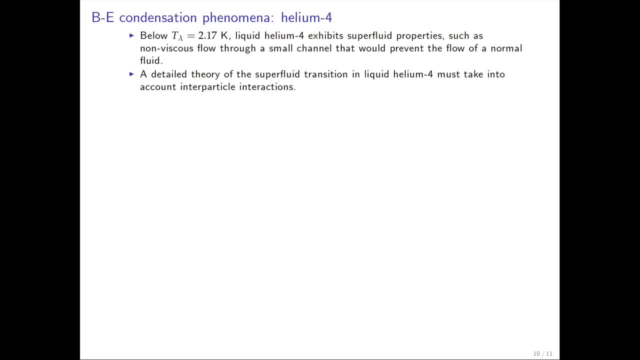 taking these nanomechanical and micro-sized resonators And now they're studying the properties of mechanical motion when it's in liquid helium and there's no viscosity. It's very interesting work. that's just happening, sort of, like I said, a rediscovery of some of liquid helium 4 effects. 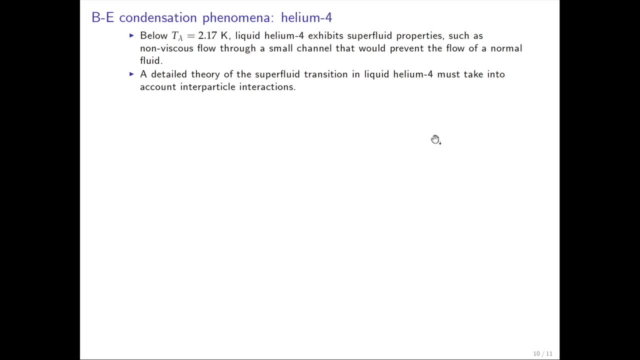 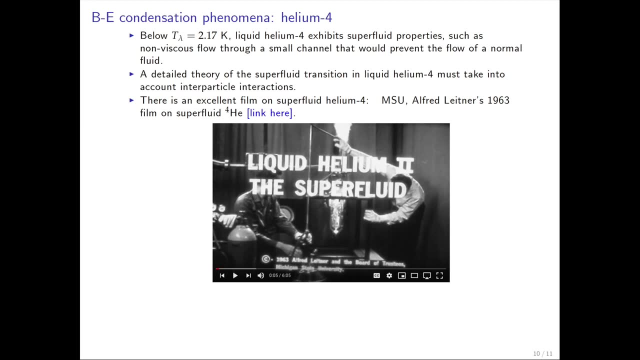 I know several people are doing it, including some in Australia. Okay, But I really want you to watch this, because you have, you're going to fall. I'm basically going to sit here going nowhere over Easter, apparently, And there is this really, really excellent film. 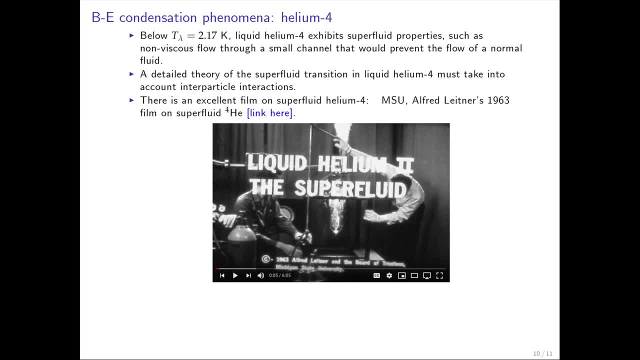 on superfluid helium-4.. It comes from the 60s, 1963, and it's this professor Offord Leitner. He was at MSU, Michigan State University, And he made this film and I remember watching this. 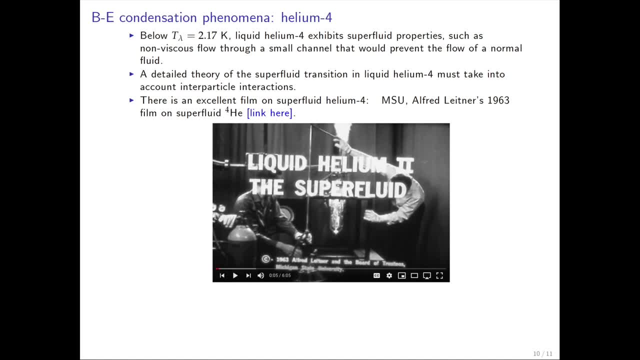 when I was an undergraduate. It totally blew me away. It was totally amazing And I put a link here. Now you can find the whole film in several parts. There's a playlist on YouTube. Let's just click it. We'll watch a little bit of it. Let's see if it will allow me to do it. 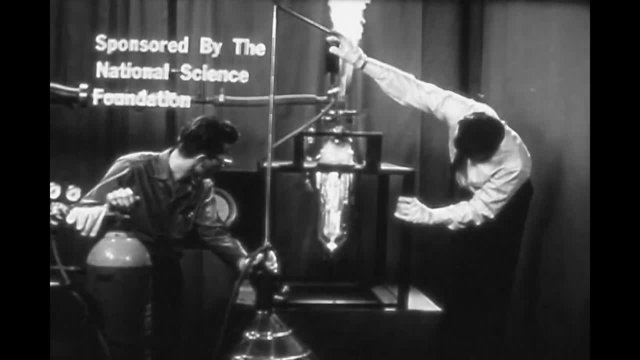 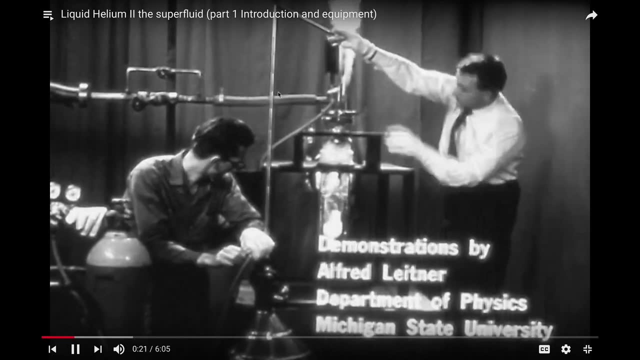 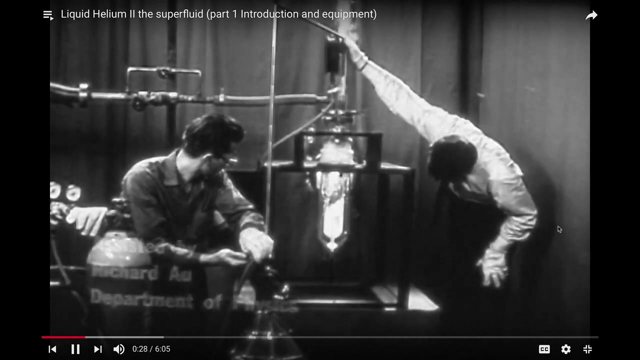 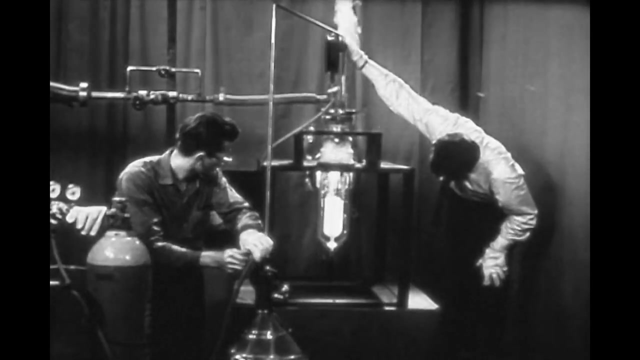 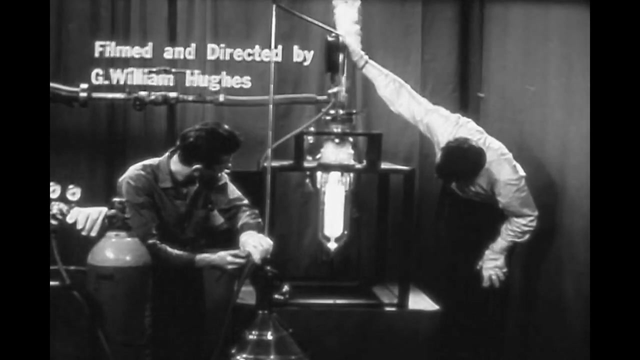 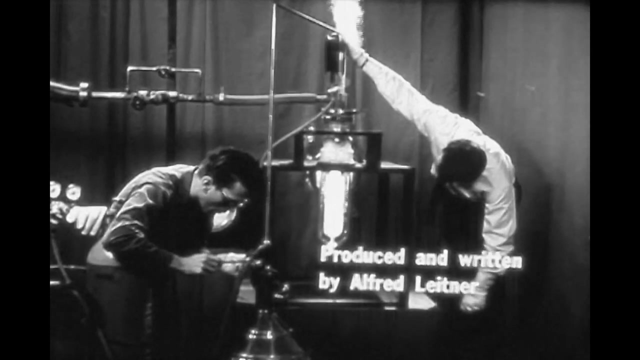 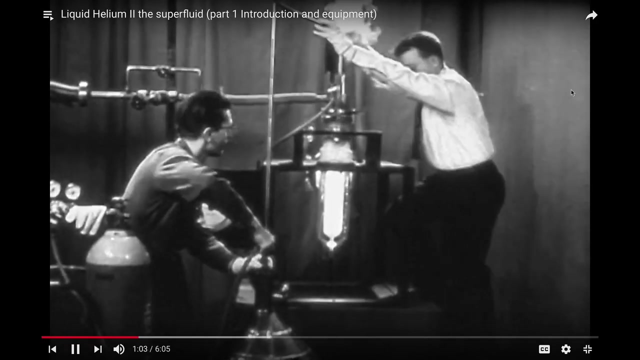 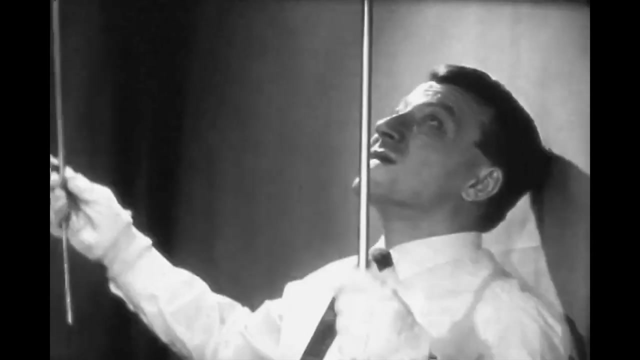 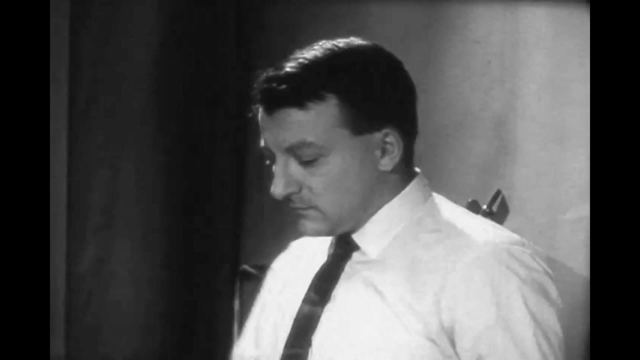 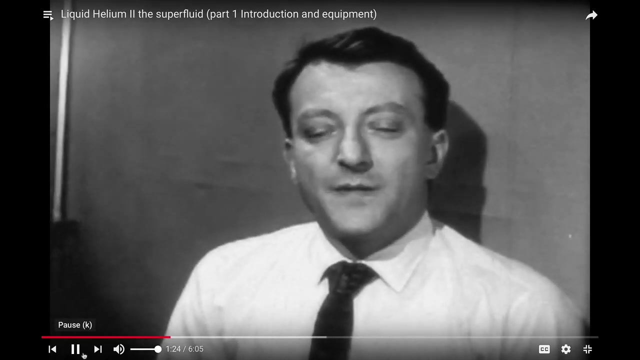 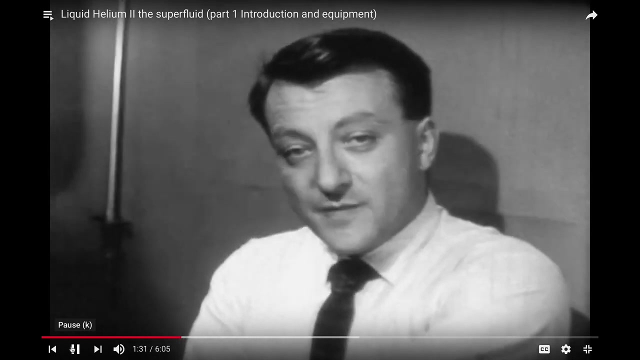 All right, To the level of the air. To the level of the air. Okay Listen, Good, Good draw. We just made a transfer of some liquid helium out of a storage tank into our own experimental equipment. Helium is a remarkable substance. It has two different and easily distinguishable. 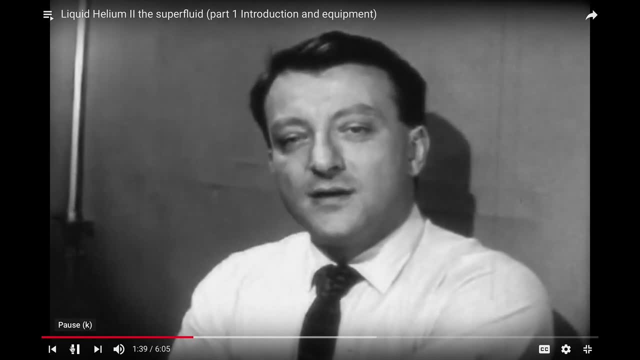 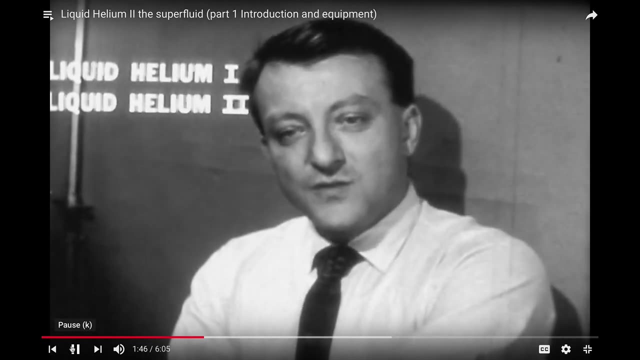 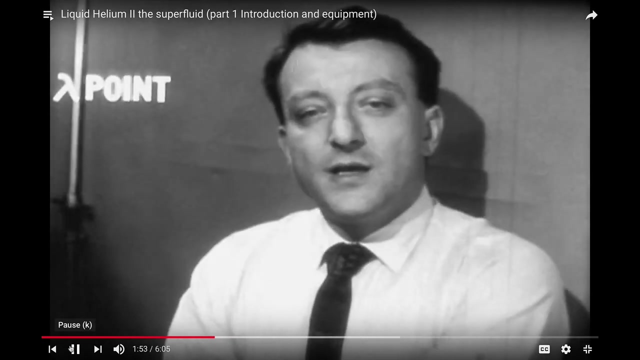 liquid phases, a warmer and a colder one. The warmer phase is called the liquid phase. It's called liquid helium-1, and the colder phase liquid helium-2.. The two phases are separated by a transition temperature, known as the lambda point. When liquid helium is cooled down through 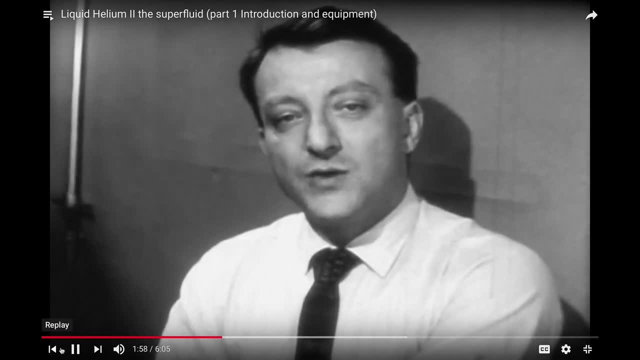 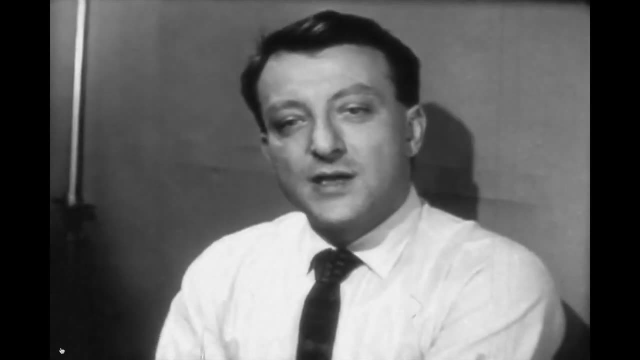 the lambda point, a transition from helium-1 to helium-2 is clearly visible. We will show it to you later in this film. The two liquids behave nothing like any other known liquids, although it could be said that helium-1 and helium-2 are the same. Helium-1,, the warmer phase, approximates the behavior of common liquids, But it is helium-2,, the colder phase, which is truly different. Because of this it is called the superfluid. The temperatures involved when working with liquid helium are quite low. Helium boils. 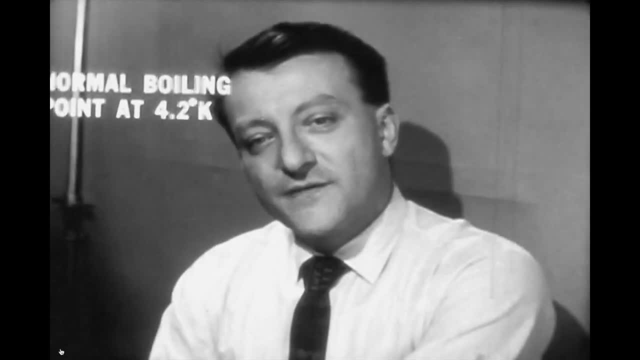 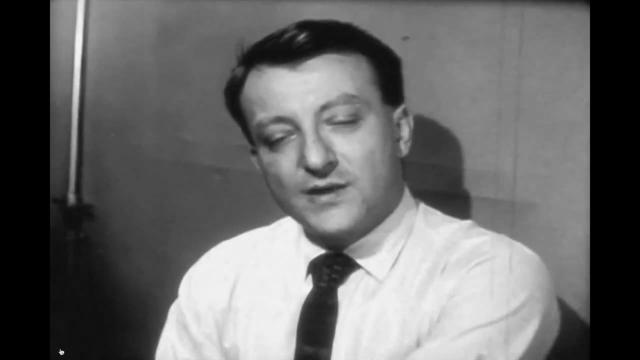 at 4.2 degrees Kelvin under conditions of atmospheric pressure and the lambda point lies at roughly 2.2 degrees. Note that this corresponds to minus 269 and minus 271 degrees centigrade. The properties of liquid helium that I have just been 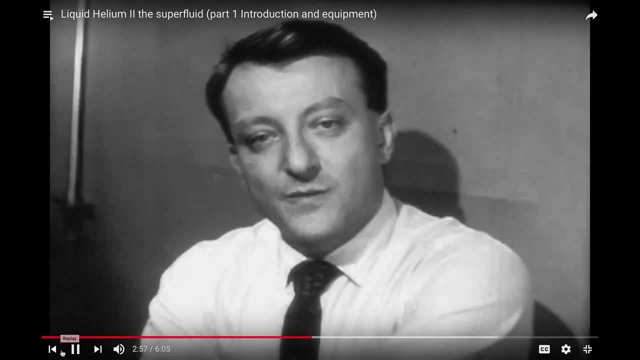 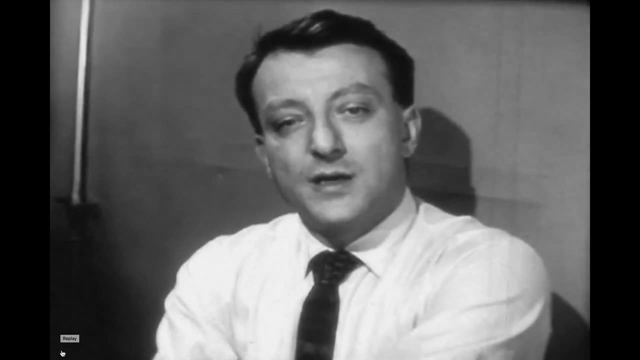 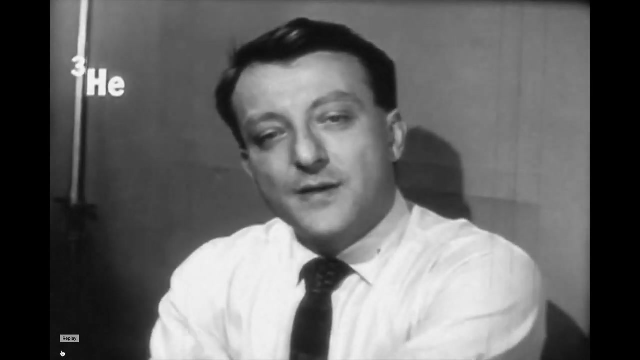 telling you about are characteristic of the heavy isotope of helium, helium-4.. The element occurs in the form of two stable isotopes. The second and lighter one, helium-3, is very rare. Its abundance is only about one part out of 10 million. Pure liquid helium-3 is the subject of intensive study at the present time, but so far no second superfluid liquid phase has been found to exist for helium-3.. Okay, did you catch what he just said there? He said no superfluid phase had been found for helium-3. 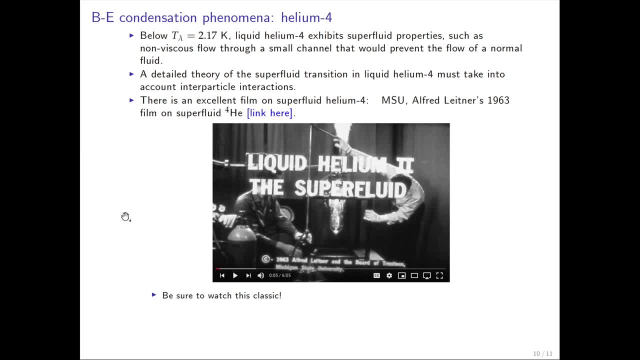 And that's because this film was made in 1963.. In fact, superfluidian helium-3 was discovered not long after that, in 1971.. So be sure to watch this. It's really great. I think you'll enjoy it. 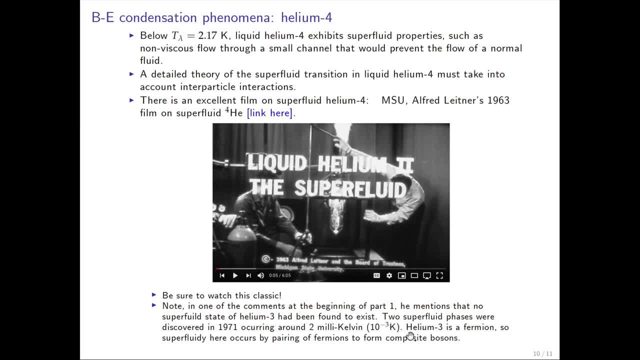 So okay, And we'll just mention that, as I said, superfluid phases: two superfluid phases actually were discovered in 1971, and they both occur around 2 millikelvin, That's 10 to the 3.. 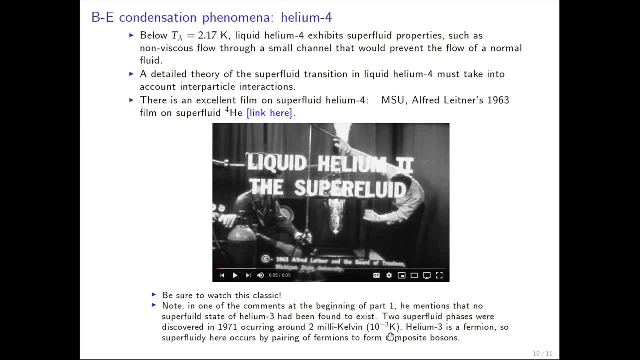 A millikelvin is 1 thousandth of a kelvin, 10 to the minus 3 kelvins. And helium-3 is a fermion, so superfluidian helium-3 occurs by pairing of fermions to form composite bosons. 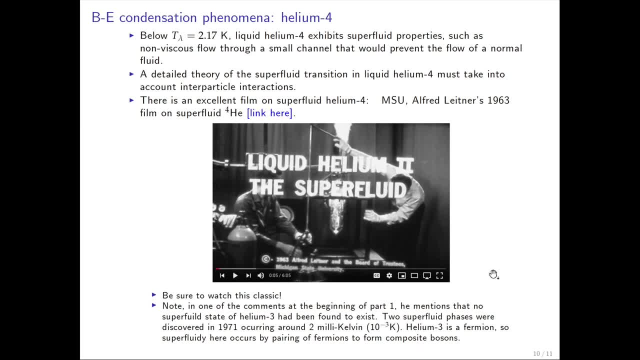 And recently I've been reading a lot about superfluid helium-3, and it's It's an incredibly complicated system. It really, I have to say, it really makes my head spin. But anyway, we'll talk about other types of condensation in the next slide. 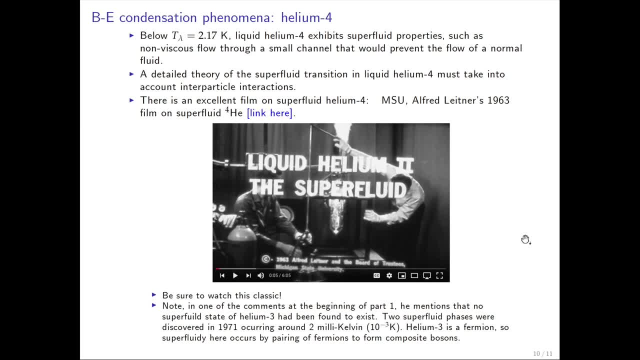 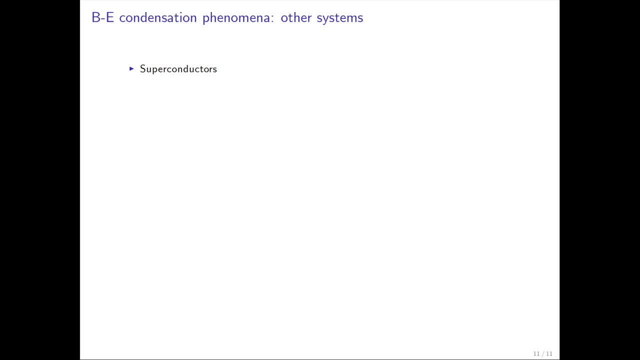 But do watch this film if you have time. I highly recommend it. Well, there are other systems, that where something like Bose-Einstein condensation is found, And of course you probably know there are things of superconductors And most elemental metals are. 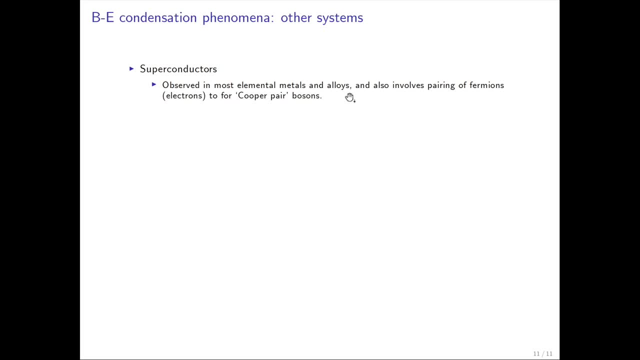 And lots of alloys are superconducted at low enough temperature, And superconductivity- the usual kind that we understand in elemental metals and alloys, and maybe In fact all types of superconductivity, involve pairing of fermions to form what are known as Cooper-Pair bosons, named after a guy named Cooper. 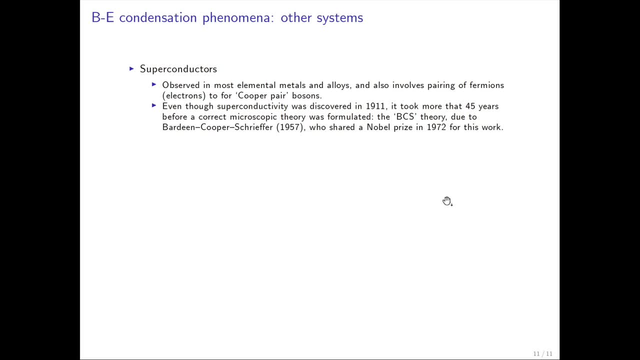 Now, superconductivity was discovered in 1911. That was by Onsaker at Sorry at, Not Onsaker. I forget the guy's name now At Leiden: Onsaker, Yes, Onsaker. 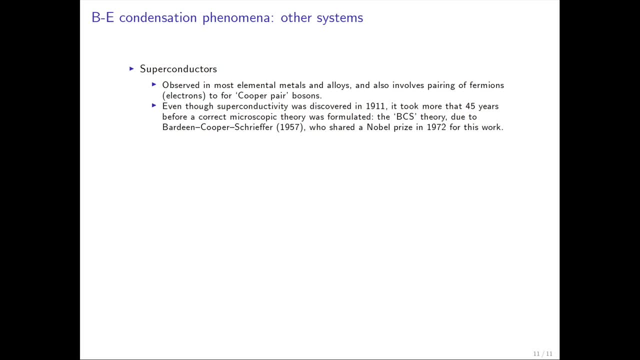 But it took more than 45 years before a correct microscopic theory was formulated that really described how fermions paired up in Cooper-Pairs and became superconducting, And this theory is known as BCS after the authors Bardeen, Cooper and Schrieffer. 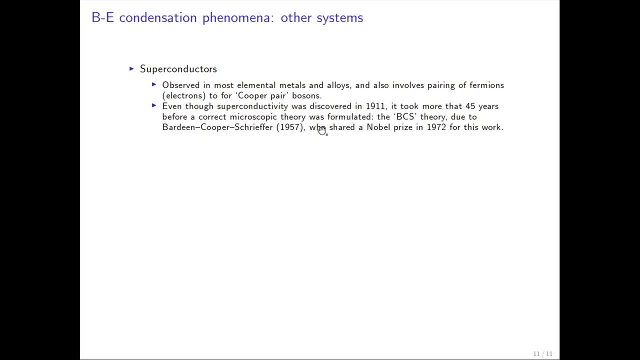 who published a paper in 1911. In 1957, about this microscopic theory, And they shared a Nobel Prize in 1972 for this work of superconductivity. So superconductivity in conventional metals is well understood in terms of BCS pairing. 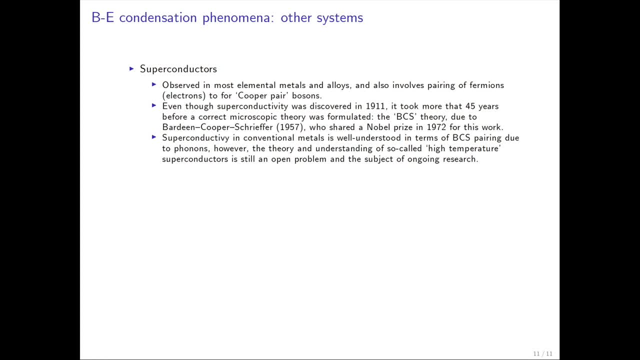 And the pairing is due to a really interesting effect when you have an effect of attraction between electrons due to phonons. However, you've probably heard, there are things called high-temperature superconductors. Starting in the mid-'80s, it was the cuprates. 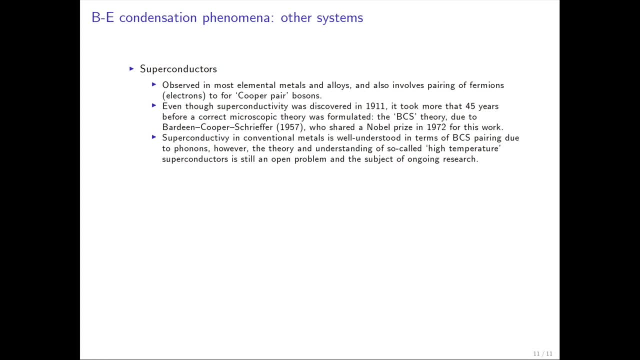 And nowadays they're. And nowadays they're the iron particulates and other materials, And these are still an open problem and subject of ongoing research. just understanding the theory, for example, And starting about in the 90s. So the history of Bose-Einstein condensation in the ideal sense was very, very long. 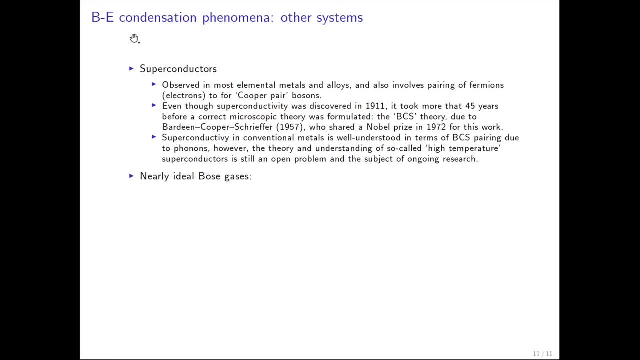 And for years people were trying to achieve a Bose-Einstein condensation that was nearly ideal And did not involve, for example, pairing like in helium-3 or superconductivity, or that was more ideal, say, than in liquid helium-4. 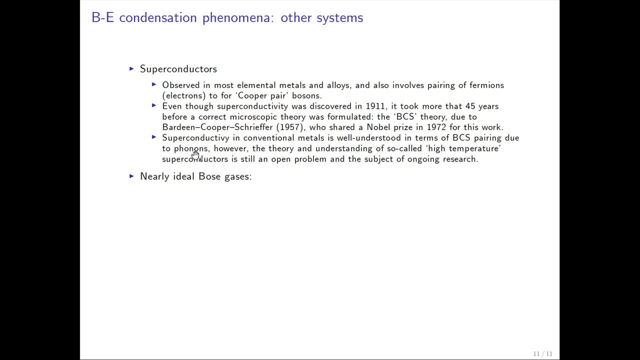 where there's strong inter-particle interactions, And so this was finally achieved, actually starting in 1995, with trapped atoms, Atoms that are trapped in magnetic traps, So that may be cool, But there are also those that can be mixed up with other atoms. 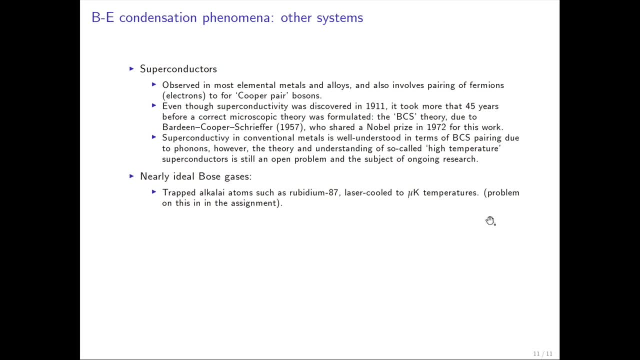 such as Rubidium-87. And they laser cool these to micro-Kelvin temperatures And there's a problem about Bose-Einstein condensation in this system. That will be, It's on your assignment- Basically this type of Bose-Einstein condensation. 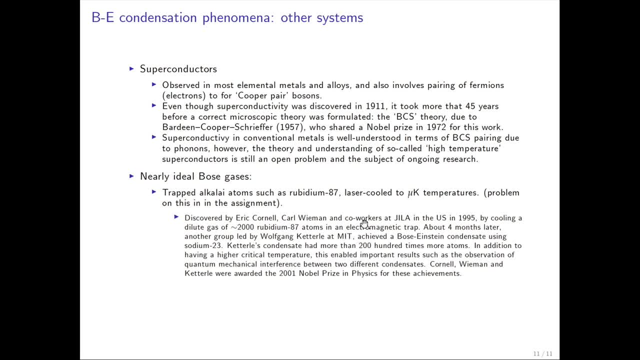 which is really truly Bose-Einstein condensation was discovered by Cornel Wieman, a joint institute in Boulder, Colorado- It's called GILA, And they discovered this in 1995 by cooling a gas of about 2,000 rubidium-87 atoms in an electromagnetic trap And about. 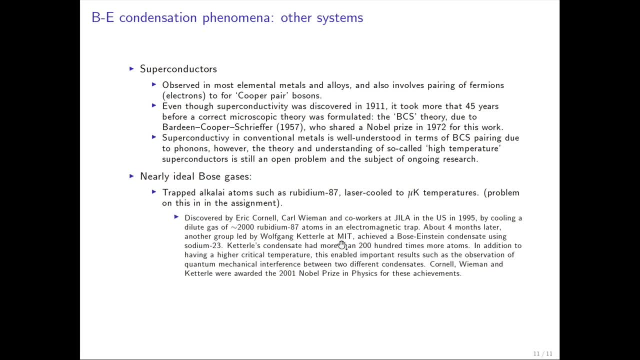 four months later another group led by Wolfgang Ketterle at MIT also achieved a Bose-Janssen condensate using sodium-23.. And Ketterle's condensate had more than something like 200 times more atoms than the 2,000 here of the Wieman's group, And of course that meant 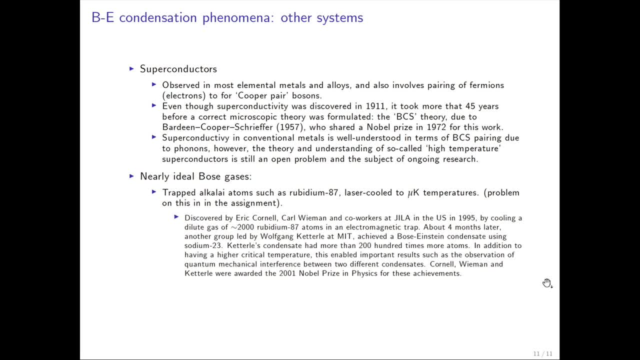 as we've seen, the critical temperature depends upon the number. So if the volume per particle is smaller, then of course the temperature can be higher And you can see the transition at a smaller de Broglie wavelength. We just argued that at the beginning of this lecture. 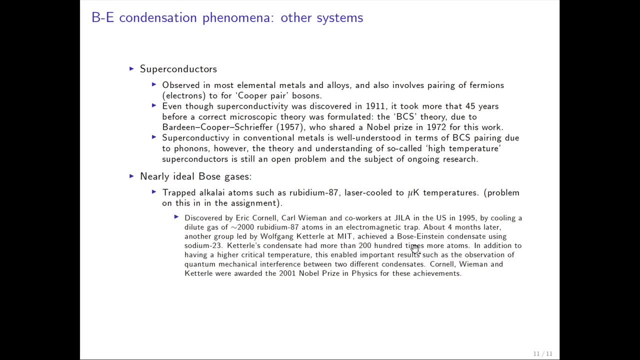 And so that's why. So getting more particles meant a higher transition temperature, And I believe the transition temperature there was- I don't remember the temperature off the top of my head, But anyway. And finally, in 1998, trapped atomic hydrogen was used. 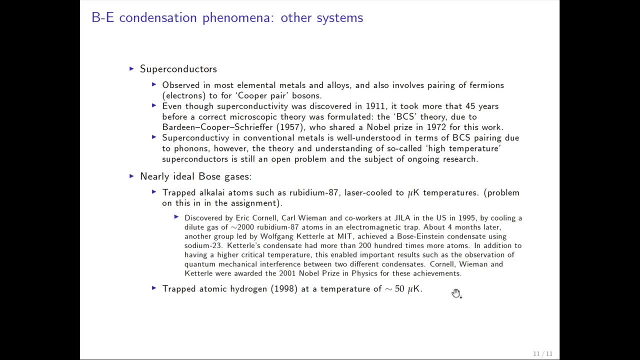 to achieve Bose-Janssen condensation at a temperature of about 50 degrees Celsius, Microkelvin- And I knew a professor myself when I was a PhD student who had worked on this for maybe over a decade. It was very difficult experimentally to achieve, And someone 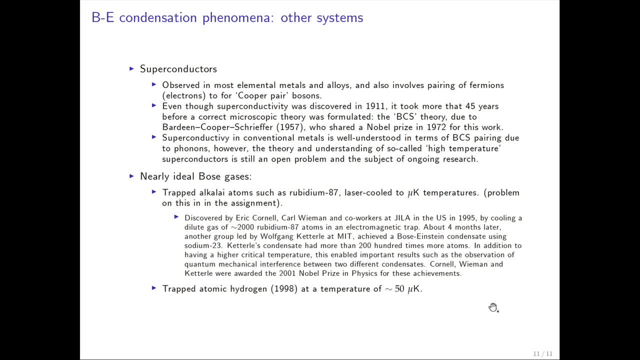 finally achieved it in 1998.. There were a number of groups racing after that, Anyway. So well, that's it for today's lecture on Bose-Janssen. It's a phenomenon, but it's very similar to the Bose-Janssen condensation and related. 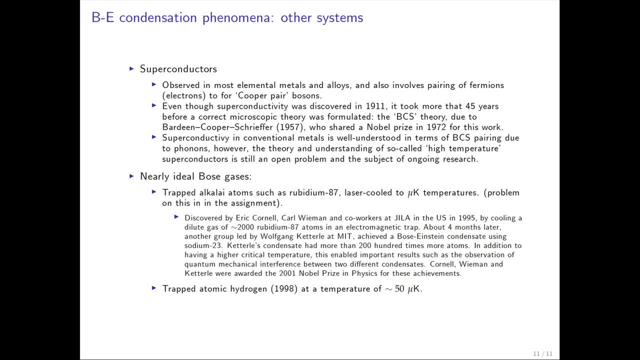 phenomenon And I'm going to. this will be your last lecture for this week, And then we'll pick up next week. when we look at, we look at photons, electromagnetic radiation in a cavity and black body radiation, And then we'll also look. finally, we'll wind.